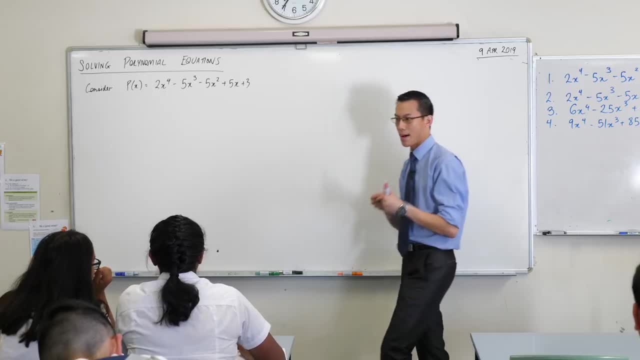 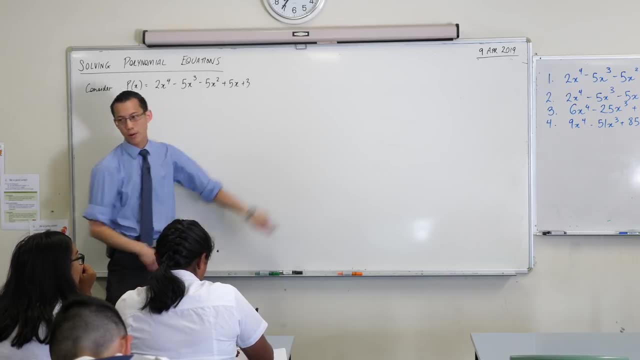 like whoa- gross and huge, but with the tools that we have at our disposal, we can totally manage these. now We can absolutely solve. if this thing were equal to zero, which is what I have over there on the right hand side- We have enough tools at our disposal to solve these, but what I would 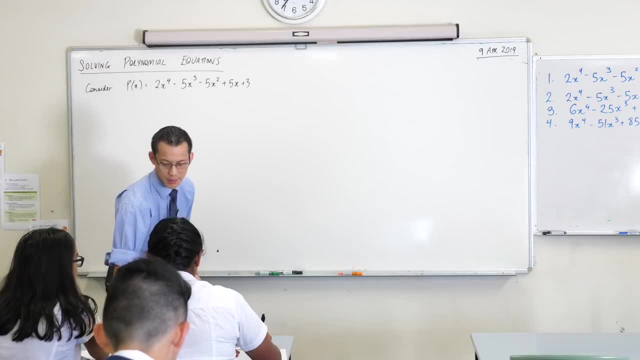 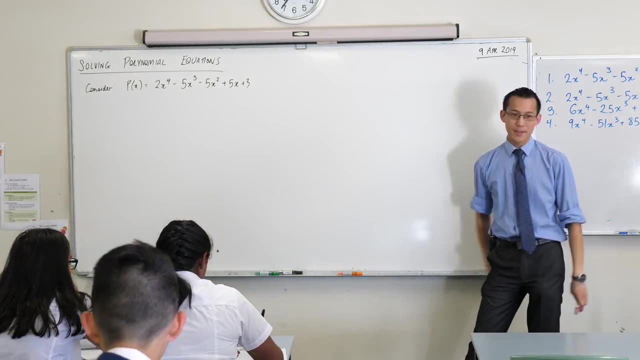 recommend- because I don't see them on every table- is: please get out your- I'm just going to pinch this. please get out your calculator, because it's going to be very handy in a second. okay, So to solve something like this, we're going to need the factor theorem. Now, if you recall yesterday, 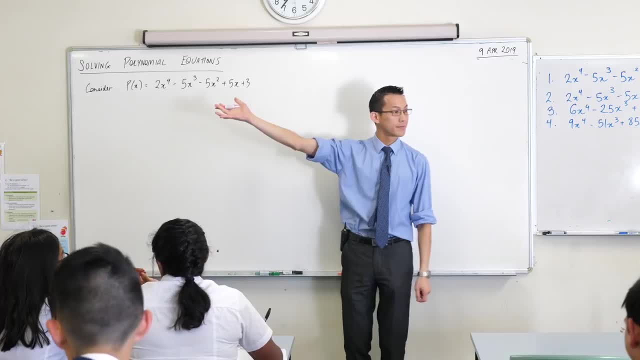 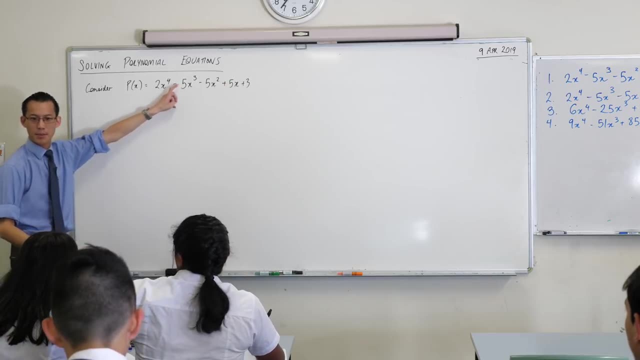 we had a look at this idea that if you have a polynomial like this, right, if you know there's going to be some factors- because, by the way, there don't always like if I gave you some weird, ridiculous numbers in here- there might not necessarily be nice factors. They might be. 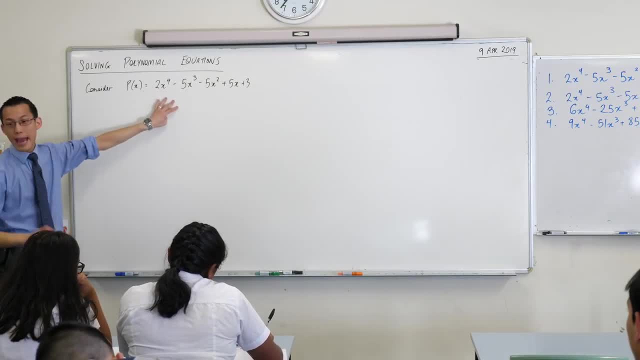 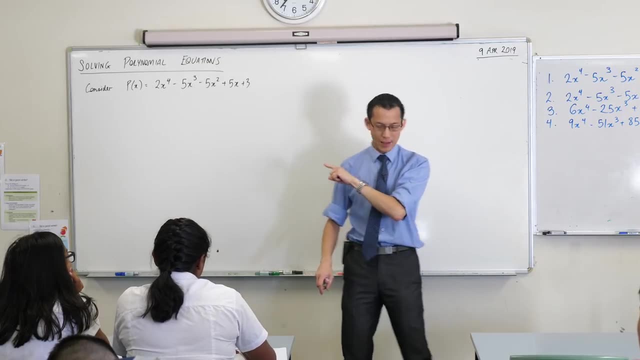 thirds, or they might be just awkward numbers- you could never guess- but we're handling ones that are quite well behaved and quite nice, and these numbers are deliberately crafted so we can factorize this thing okay. So where we're going to be headed is something like this: It's a quartic. 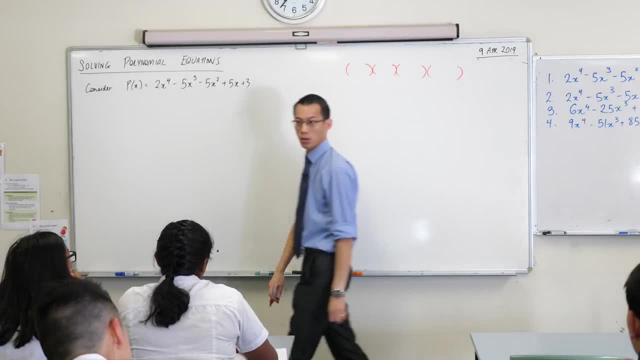 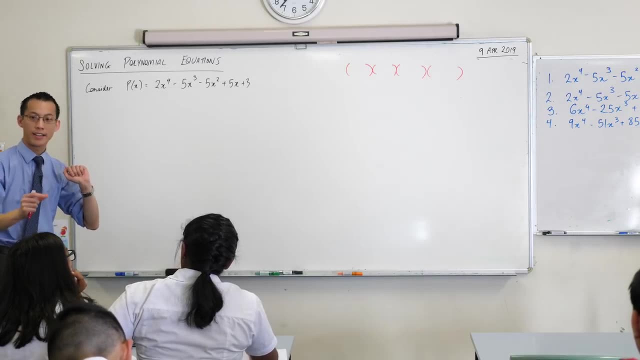 so we're going to have four factors. all along the way here right Now, we learned that if we want to find these factors, we can actually do a little bit of trial and error to work out what this thing might factorize into. For example, if we tried, say, a number of numbers and we're going to have 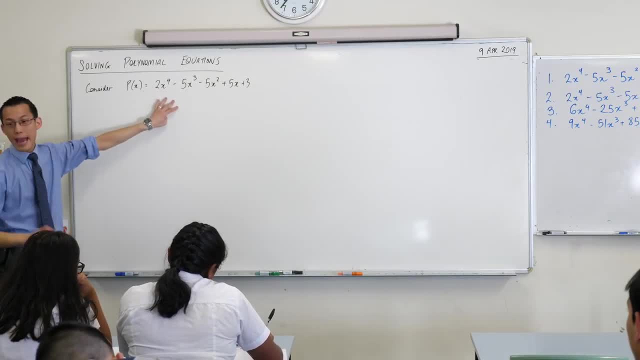 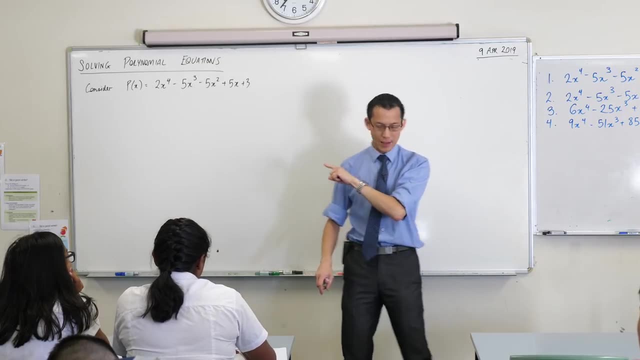 thirds, or they might be just awkward numbers- you could never guess- but we're handling ones that are quite well behaved and quite nice, and these numbers are deliberately crafted so we can factorize this thing okay. So where we're going to be headed is something like this: It's a quartic. 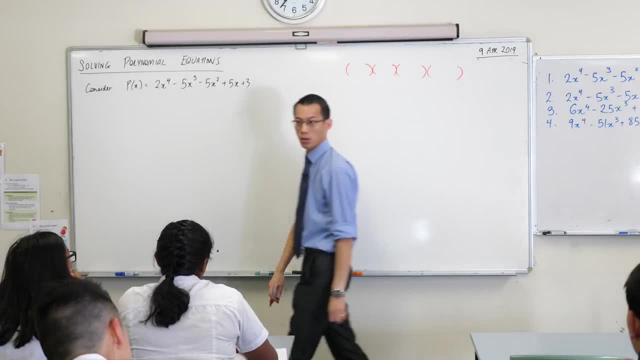 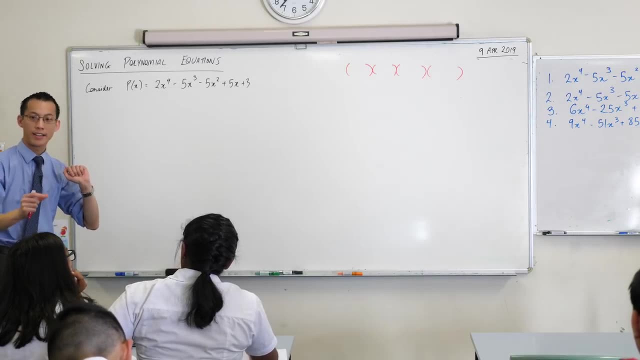 so we're going to have four factors. all along the way here right Now, we learned that if we want to find these factors, we can actually do a little bit of trial and error to work out what this thing might factorize into. For example, if we tried, say, a number of numbers and we're going to have 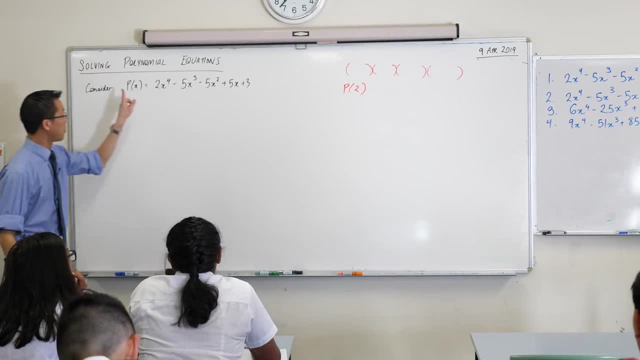 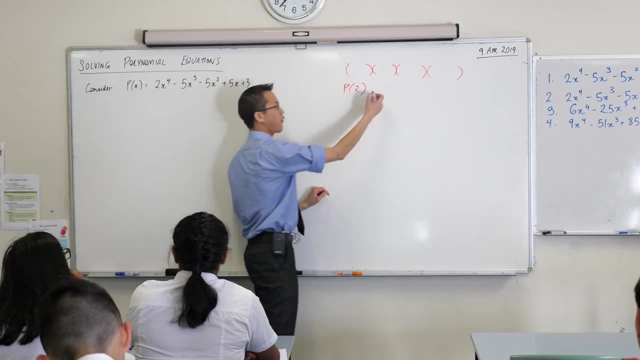 a p of two. This is the polynomial p of x, right. If we substituted two into all of this, if, for example, I'm 99% sure it's not, but if, for example, we evaluated that in our calculator and we got. 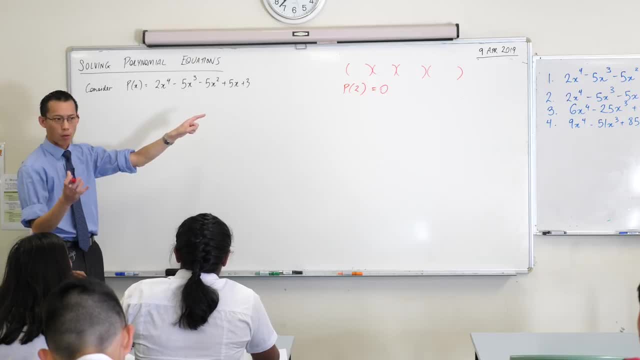 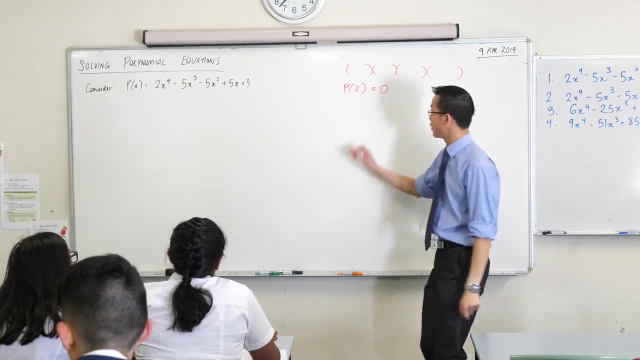 zero, then the factor theorem tells us what. What is a factor of this? if we can see this is true, Who remembers from yesterday X minus two? very good, If I see this, I would literally write on the next line. 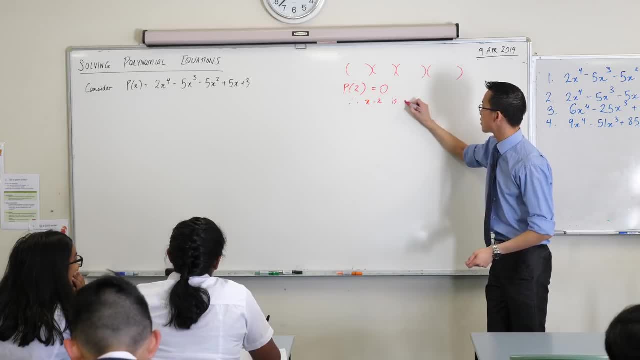 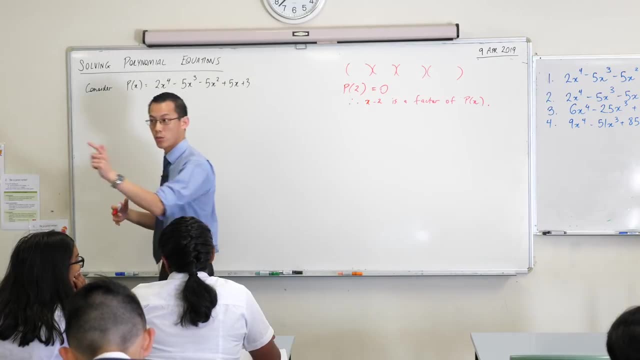 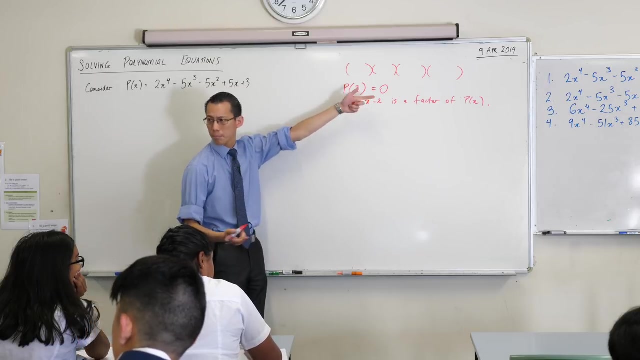 after this I would say: therefore, x minus two is a factor of the original polynomial, And then I can divide through. by that, I'll get a cubic and it'll be easier to work with Rastan. Okay, so if you're trying to think about why, is this a minus sign and not a like a plus, like this: 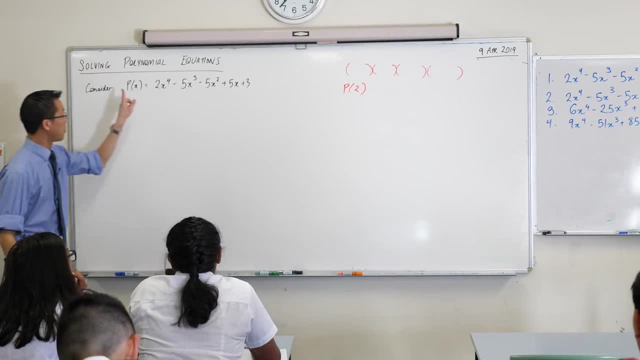 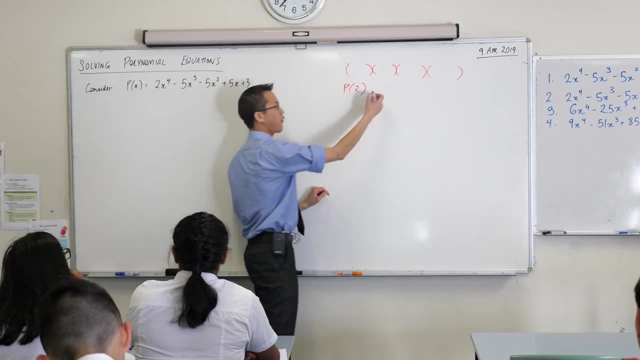 a p of two. This is the polynomial p of x, right. If we substituted two into all of this, if, for example, I'm 99% sure it's not, but if, for example, we evaluated that in our calculator and we got. 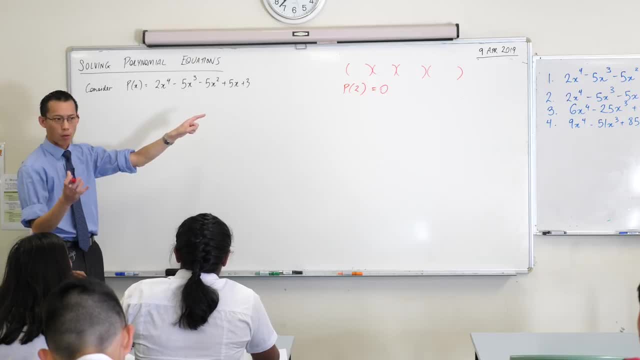 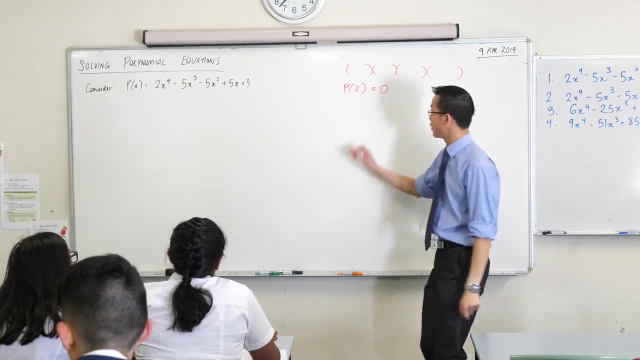 zero, then the factor theorem tells us what. What is a factor of this? if we can see this is true, Who remembers from yesterday X minus two? very good, If I see this, I would literally write on the next line. 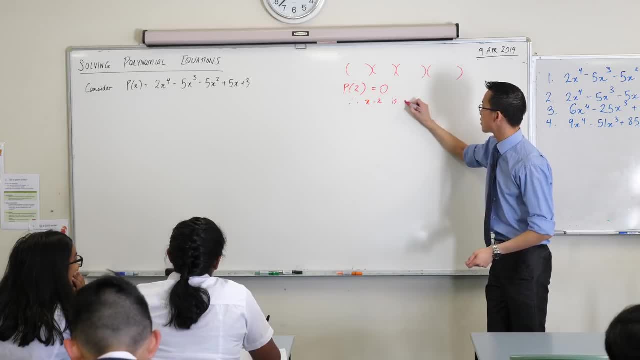 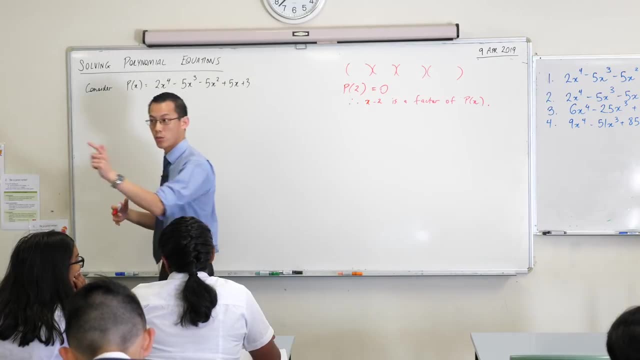 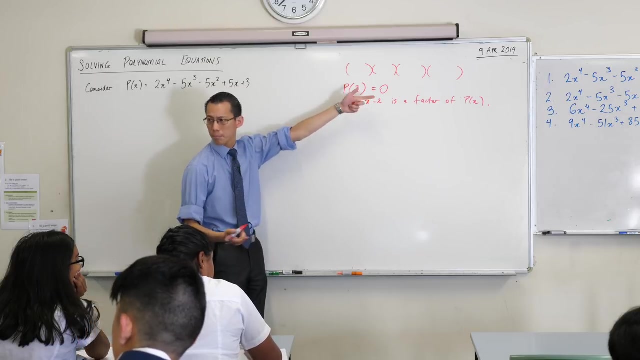 after this I would say: therefore, x minus two is a factor of the original polynomial, And then I can divide through. by that, I'll get a cubic and it'll be easier to work with Rastan. Okay, so if you're trying to think about why, is this a minus sign and not a like a plus, like this: 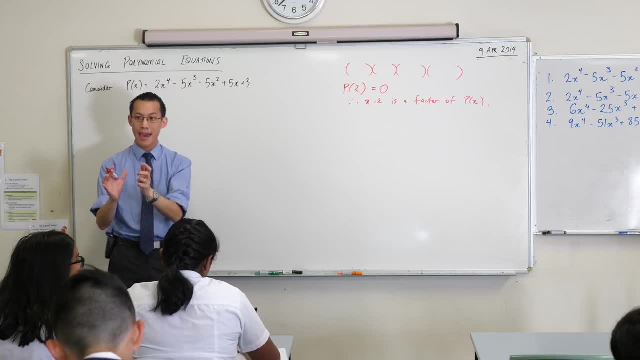 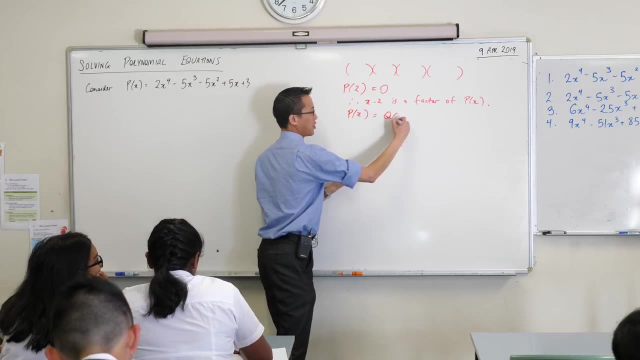 is plus. why is this not plus? I want you to go back to that statement we made from. after you do a long division, you would say: your original polynomial is equal. to think back right, Your quotient and fact we can figure out. if that's the answer, You forget the point On the c. you wouldn't even know. 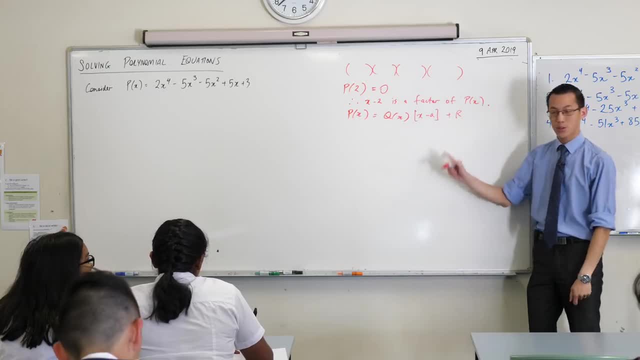 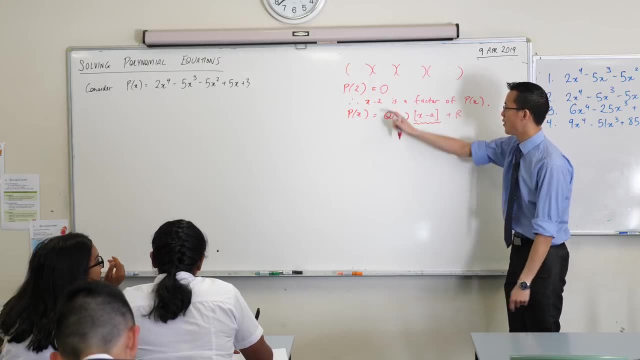 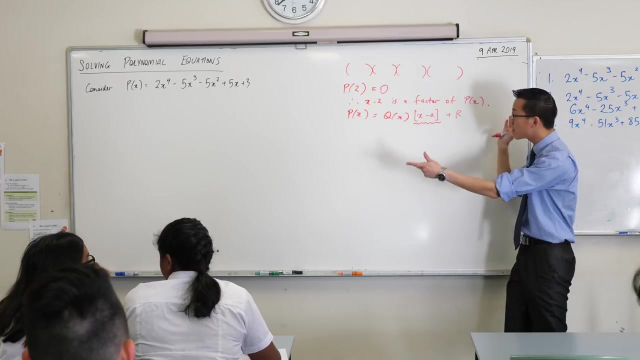 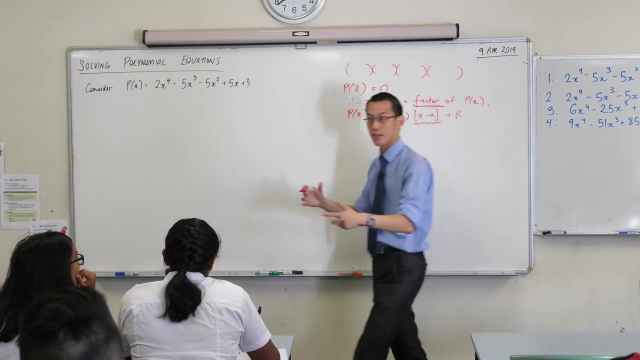 what you're doing, What Wi purposely couldn't answer. you'd say you're replacing this with even by keeping this stepping. But then what is the next step? Take the second Mean, specify the first and the third possible MI length carriers. The third and final plaster of the Neither is that. 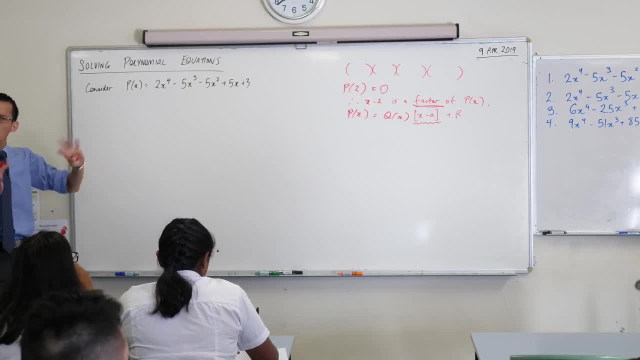 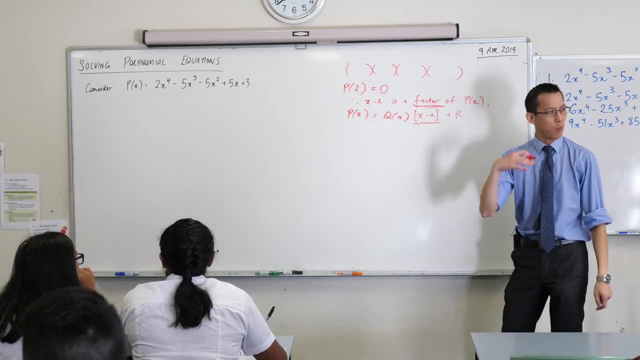 this is where we're headed right Now. what we want to end up with is something where you've got all of these bits and pieces all factorised, all nice and neat. Now I just want you to think about what it might actually do, because 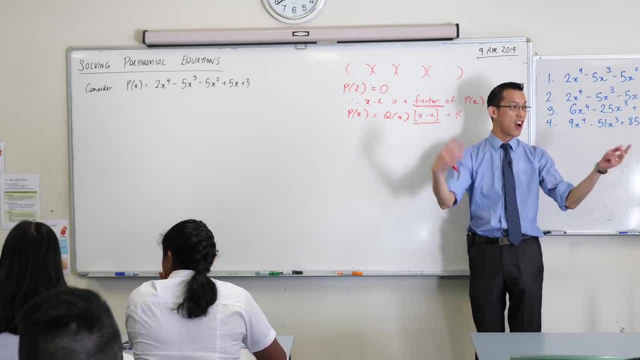 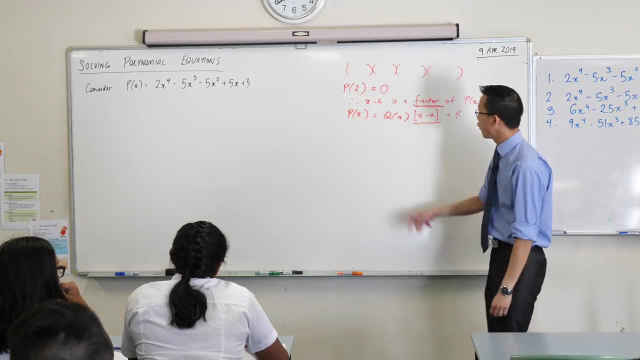 we can guess at these, right. I could just try 2,, I could try 19,, I could try 8. but you actually can use a little bit of logic to not just randomly guess. okay, For example, let's just suppose I'm just going to make up a. 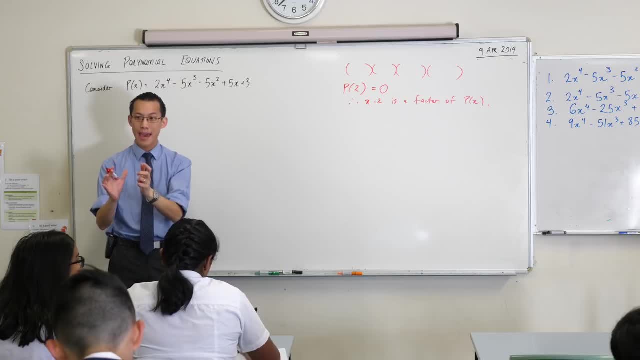 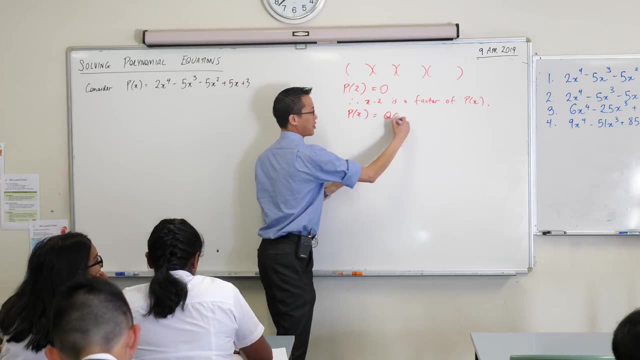 is plus. why is this not plus? I want you to go back to that statement we made from. after you do a long division, you would say: your original polynomial is equal. to think back, right? Your quotient and multiplier is zero, right? And I just have to write it down. I don't know why you feel that way. 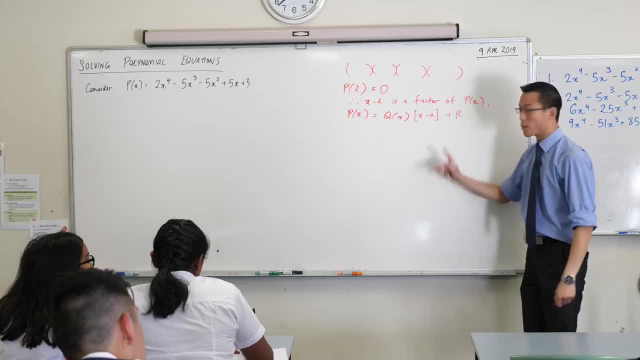 Well, I really like that In a particular way that I stated it was to have this as our divisor, this guy in here, right? The reason why was so that if you put in a into here, like, say, for example, two, 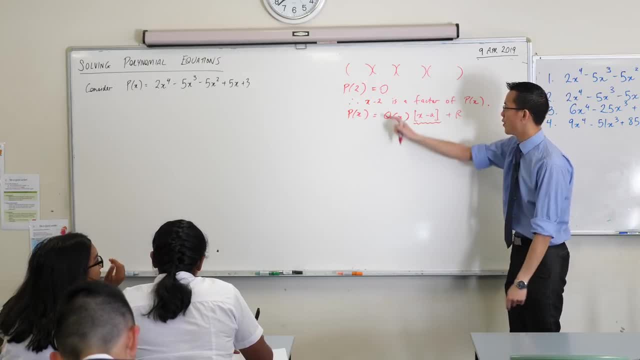 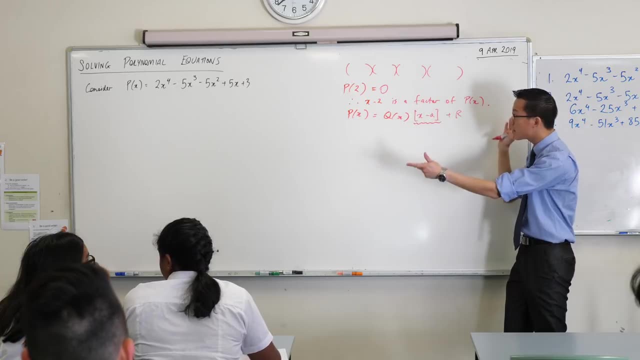 that's what makes this thing disappear, okay. So putting two into here makes this zero, which is what makes this part disappear. You just get the remainder, okay. So that was the remainder theorem, And this is that particular example where the remainder was zero. You're like cool, that means it's. 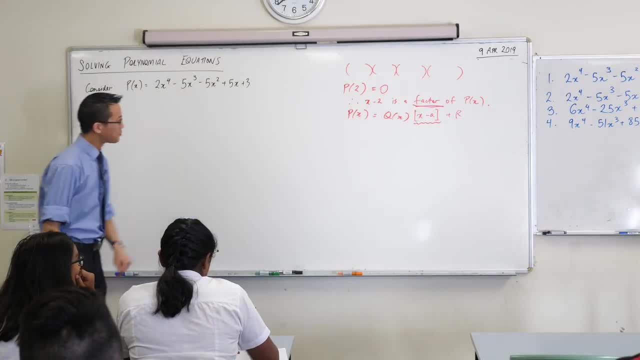 not just any old divisor, it's a factor. Okay, So right here, you've already found out this divisor and this divisor, As we've seen, this divisor and this divisor. this is where we're headed right now. what we want to end up with is something where you've got all 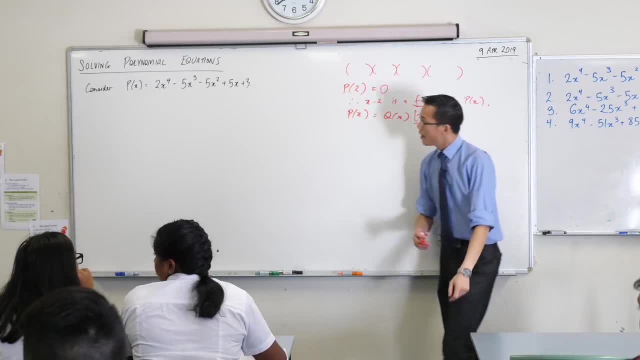 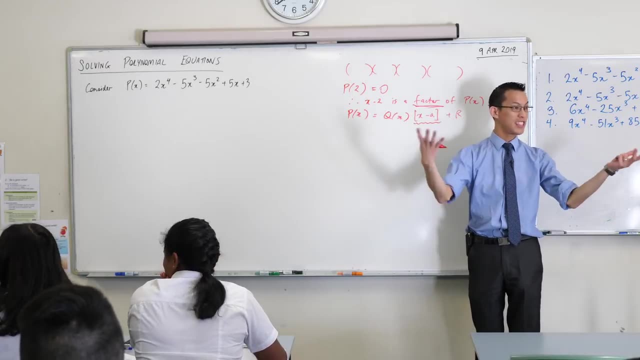 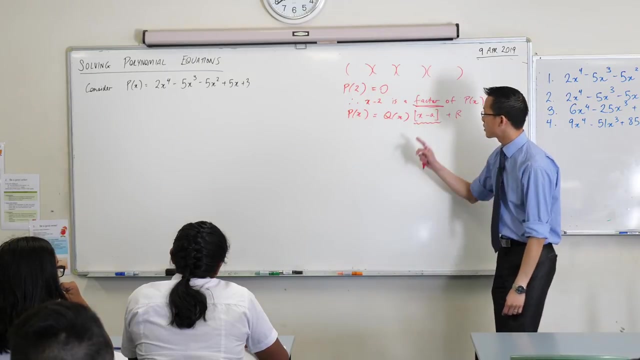 of these bits and pieces, all factorized, all nice and neat. now i just want you to think about what it might actually do, because we can guess at these, right, i could just try two, i could try 19, i could try eight. but you actually can use a little bit of logic to not just randomly guess, okay. for example, 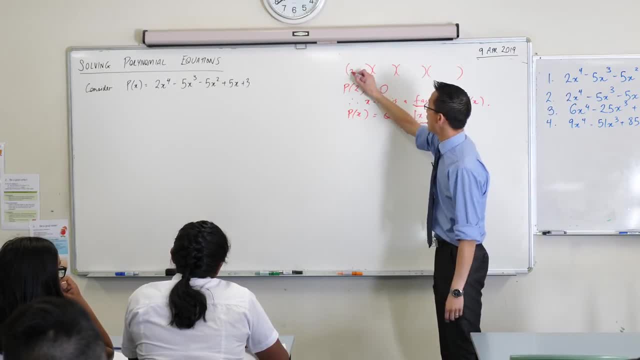 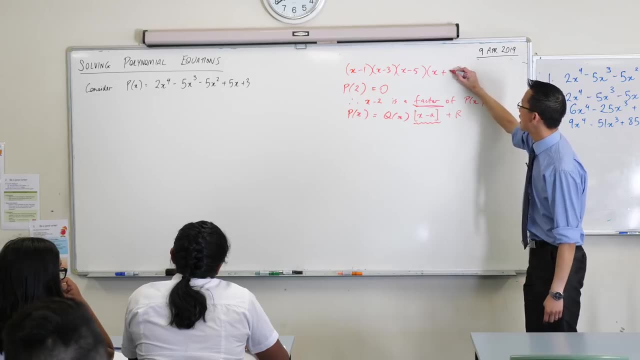 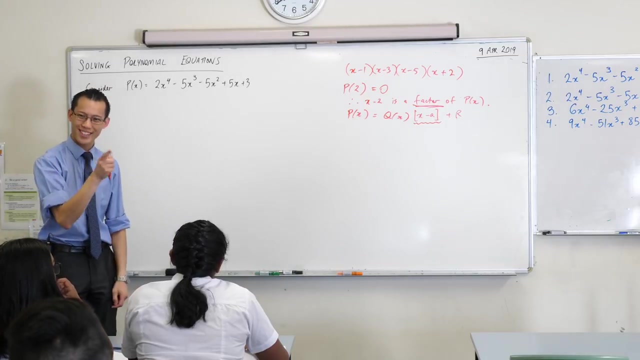 um, let's just suppose i'm just going to make up a polynomial right now. if i had a polynomial like this, uh, let's make that two on the end. okay, now i'm not actually going to ask you to expand this whole thing. i'm just interested in when i do expand it, when i'm finished. right, there's going. 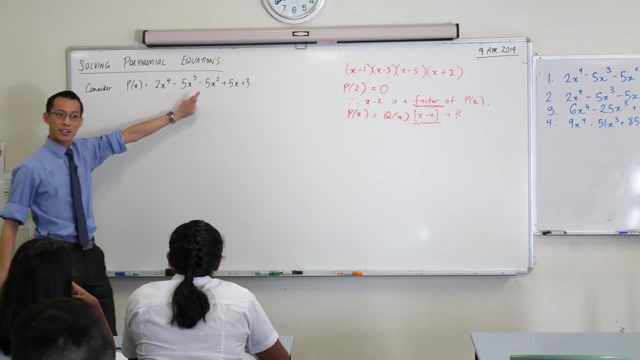 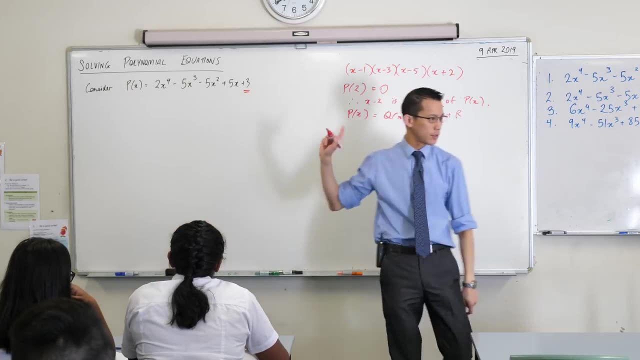 to be an x to the four term. there's going to be an x cubed term, an x squared term and an x term, and there will also be a constant term, and this constant term is actually the thing i'm interested in. just have a look at this right when this whole thing is expanded. 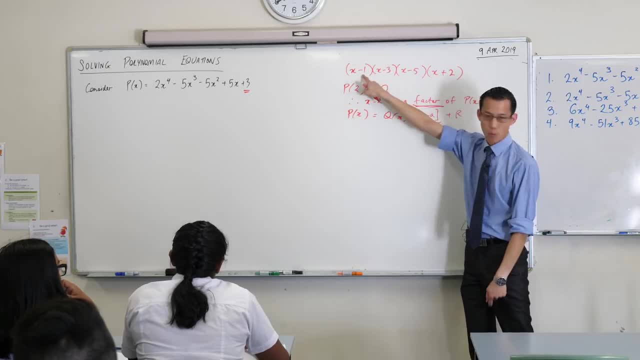 you, You're going to do x times all of these and you're going to do negative 1 times all of these. Then you're going to do x times all of these and negative 3 times all of these, And you're going to do that. 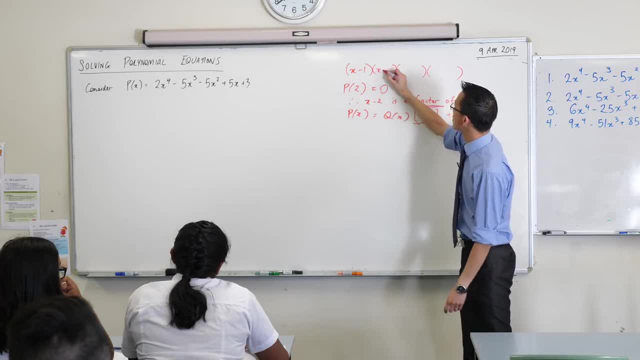 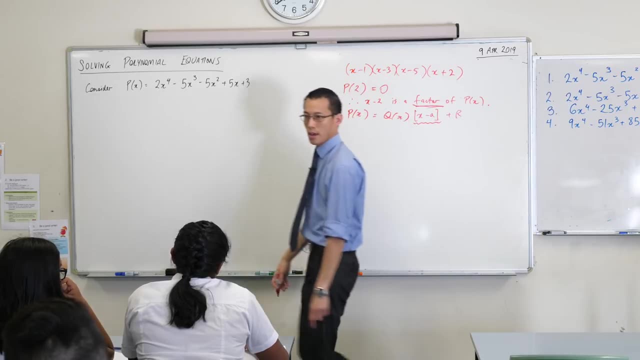 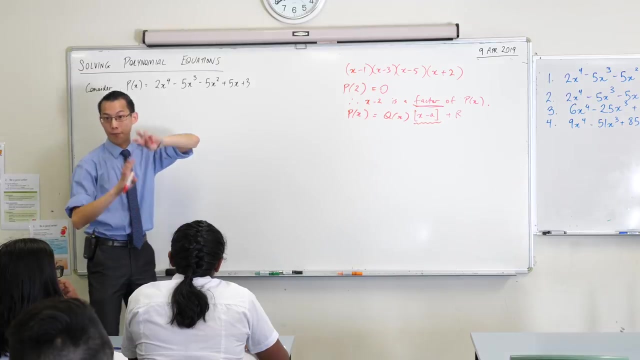 polynomial right now. If I had a polynomial like this, let's make that 2 on the end. okay, Now I'm not actually going to ask you to expand this whole thing. I'm just interested in when I do expand it when I'm finished, right? 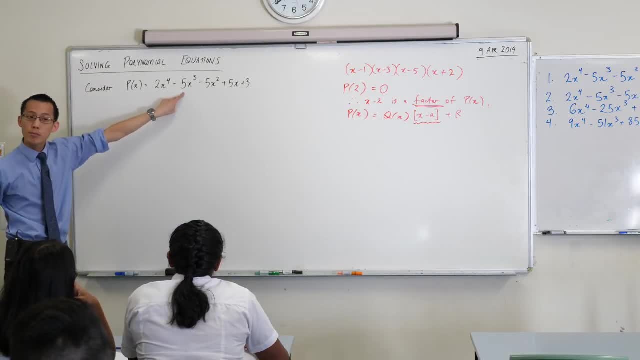 There's going to be an x to the 4 term, there's going to be an x cubed term, an x squared term and an x term, and there will also be a constant term, and this constant term is actually the thing I'm. 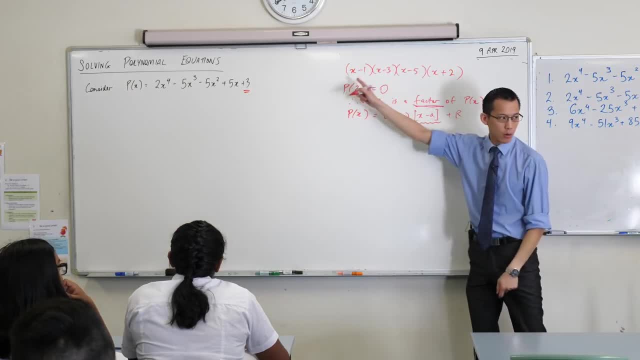 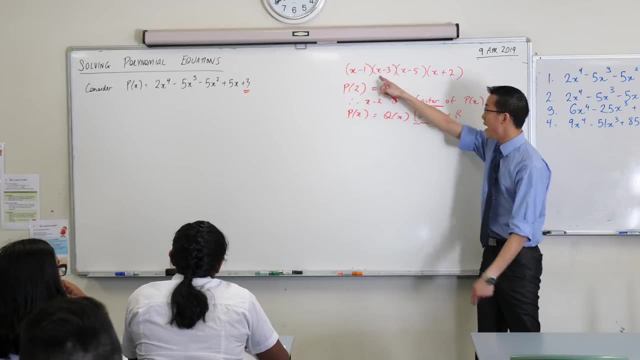 interested in. Just have a look at this right, When this whole thing is expanded, you're gonna do x times all of these and you're gonna do negative 1 times all of these. then you're going to do x times all of these and negative 3 times all of. 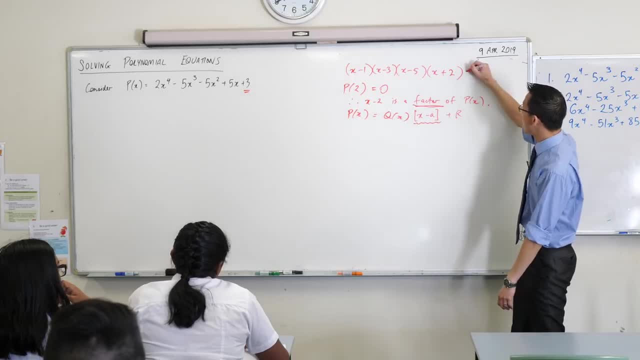 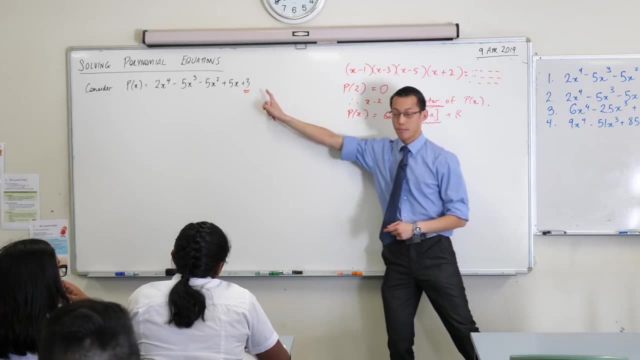 these and you're going to do that. it's going to take a long time because there are so many factors, right, But I can say with confidence that, after you've done all of that expansion, that constant term, this one on the end- is going to be equal to. 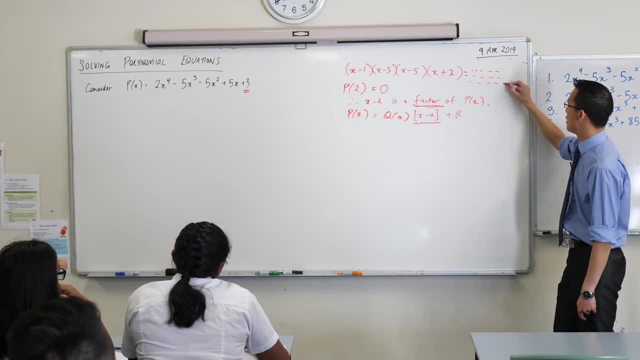 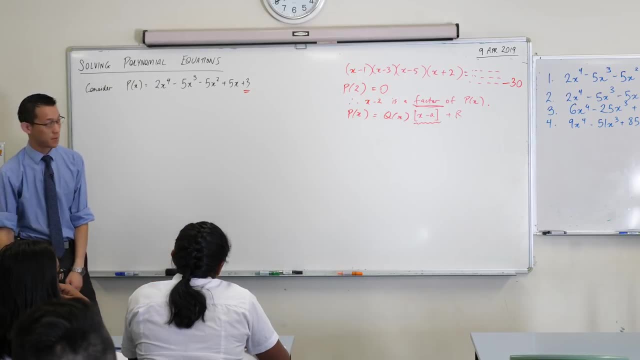 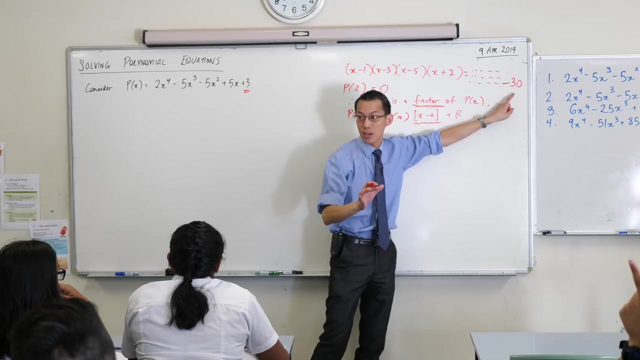 exactly negative 30. Now I wonder if anyone can tell: without me having having expanded, I literally have no idea what the rest of the terms are right. Without me having gone through that long process, how could I immediately know that the very last term we negative 30?? 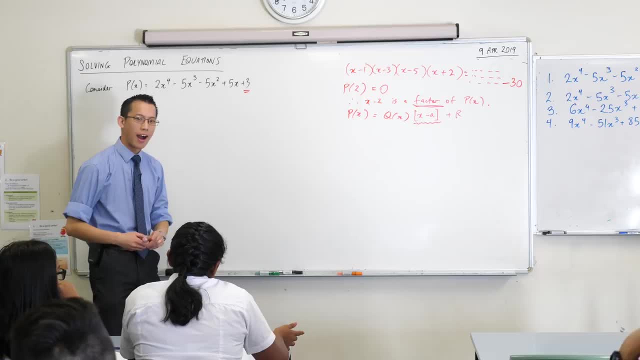 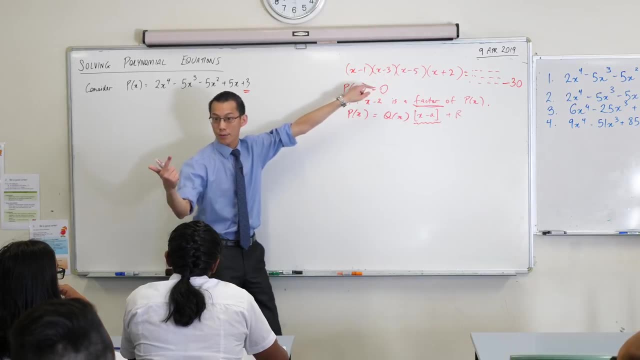 What do you say? Right, I just multiplied. Which things did I multiply All of these guys here? right, I went negative 1, negative 3,, negative 5, and then plus 2.. Is that negative 30? It is right. 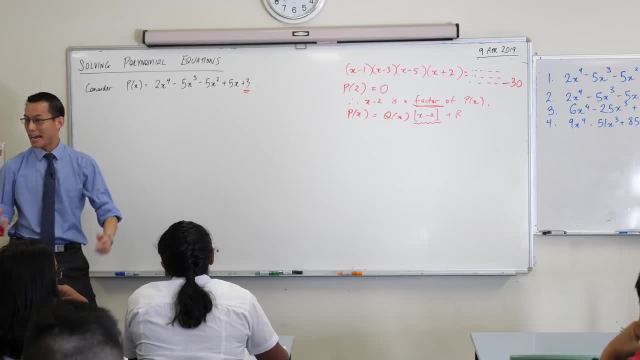 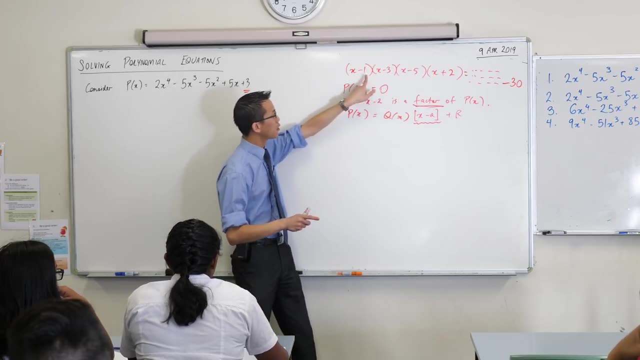 Okay, good, I can still do my numbers right Now. the reason I know that that's going to be your final term is the only time you're going to get a constant out of all of these together is when you're multiplying these guys, right? 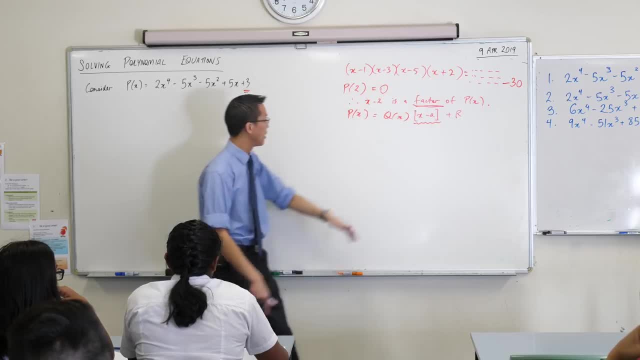 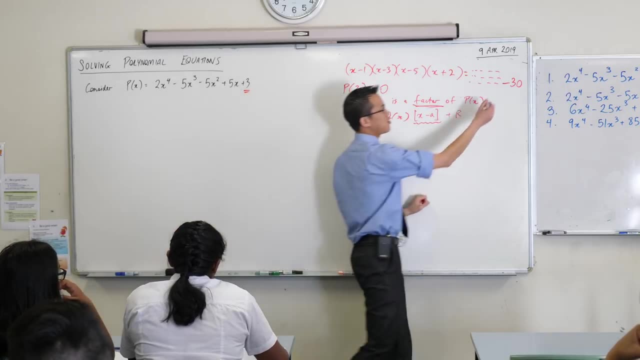 As soon as you add in one of the x's from any of those factors, you're going to get one of these right, And so I'm going to have x's in there. It won't be part of the constant. So, as a consequence, when you look at this right, 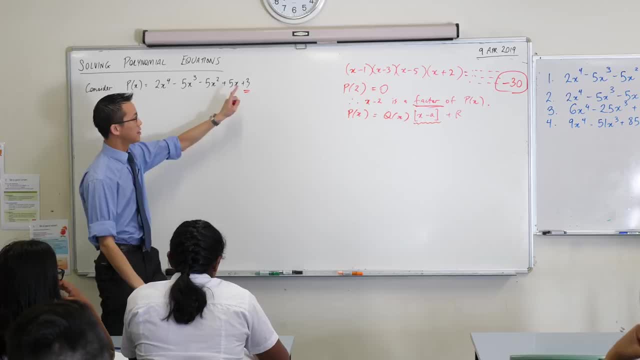 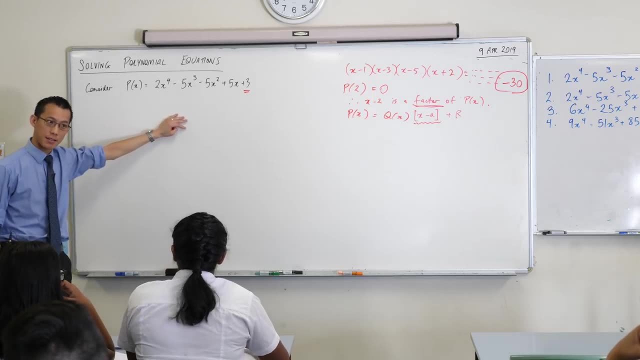 it gives you clues immediately as to what the factors must have come from. So have a look right. See how there's a 3 there. There's a 3 on the end. So I have a really good guess that either 3 or negative 3,. 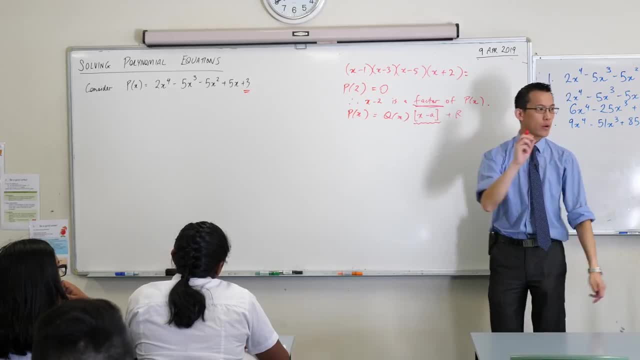 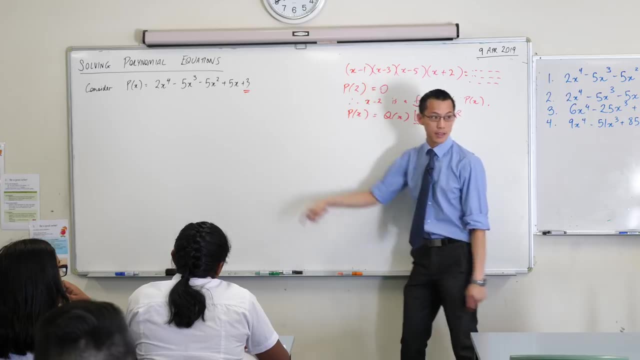 It's going to take a long time because there's so many factors, right, But I can say with confidence that after you've done all of that expansion, that constant term, this one on the end, it's going to be equal to exactly negative 30.. 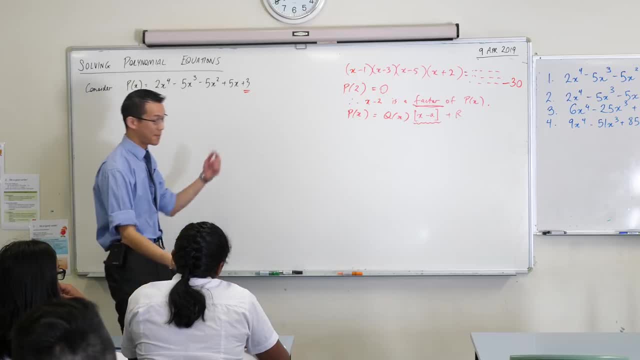 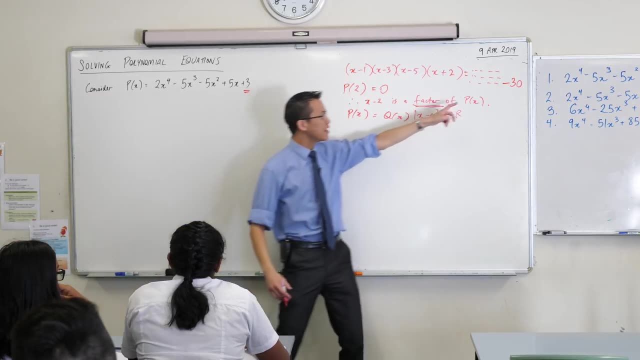 Now I wonder if anyone can tell without me having expanded any. I literally have no idea what the rest of the terms are right. Without me having gone through that long process, how could I immediately know that the very last term we negative 30?? 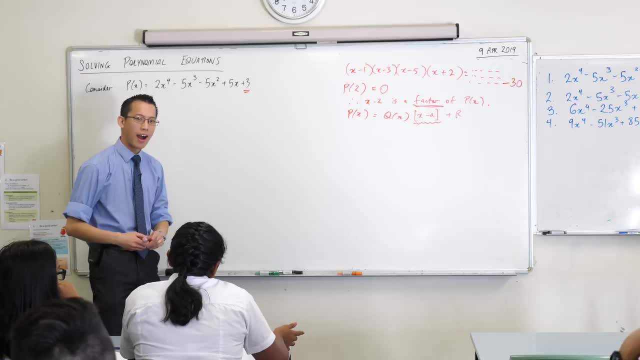 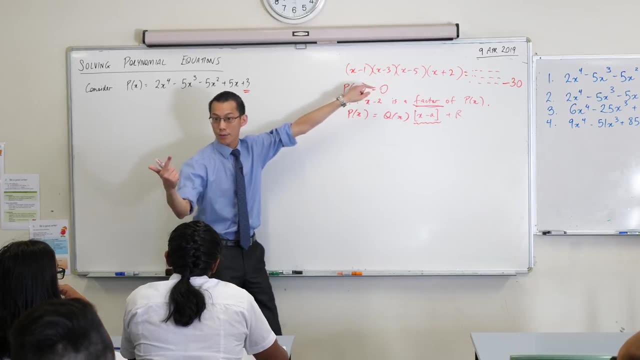 What do you say? Right, I just multiplied. Which things did I multiply All of these guys here? right, I went negative 1, negative 3, negative 5, and then plus 2.. Is that negative 30?? 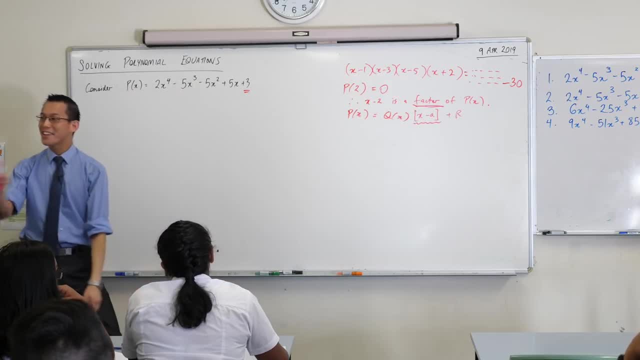 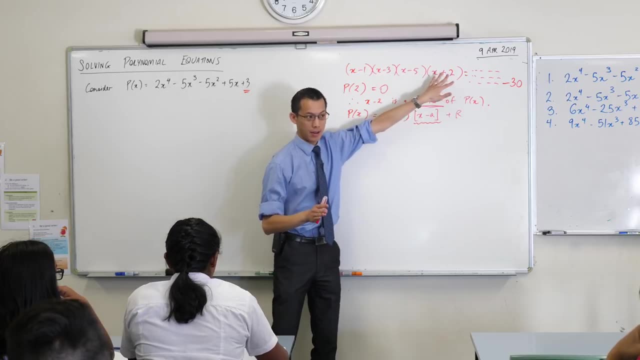 It is right. Okay, good, I can still do my. I can still do my numbers right Now. the reason I know that that's going to be your final term is the only time you're going to get a constant out of all of these together. 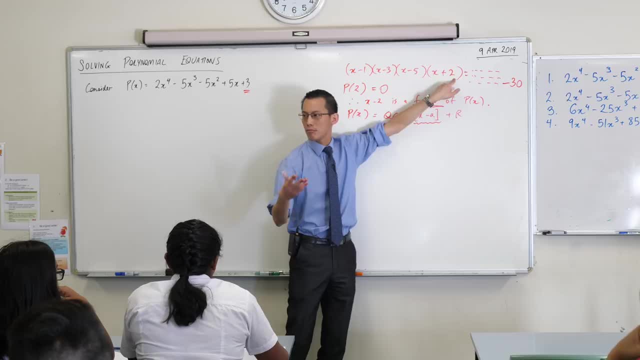 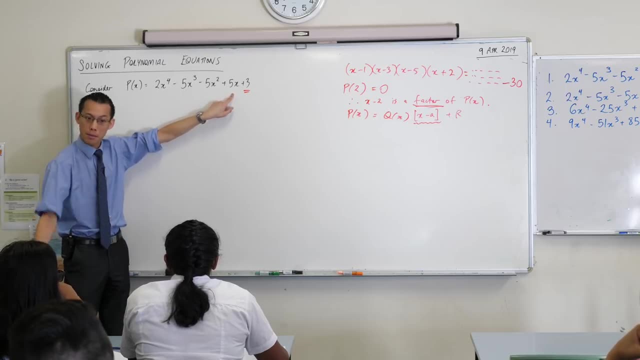 is when you're multiplying these guys right. As soon as you add in one of the x's from any of those factors, you're going to get one of these right, And so I'm going to have x's in there. It won't be part of the constant. 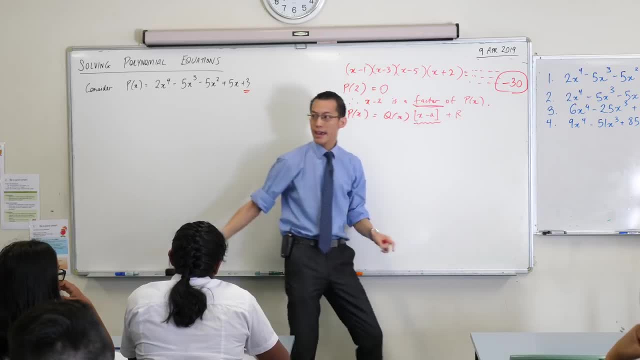 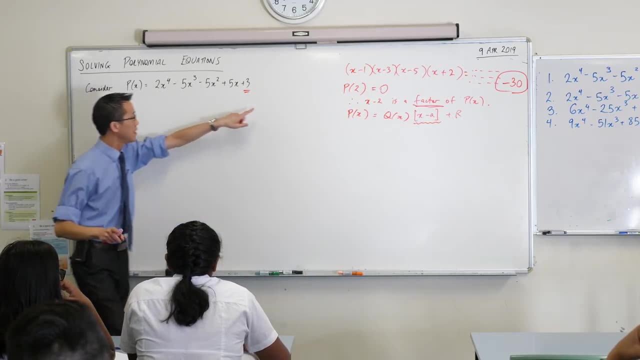 So, as a consequence, when you look at this right, it gives you clues immediately as to what the factors must have come from. So have a look. See how there's a 3 there. There's a 3 on the end. 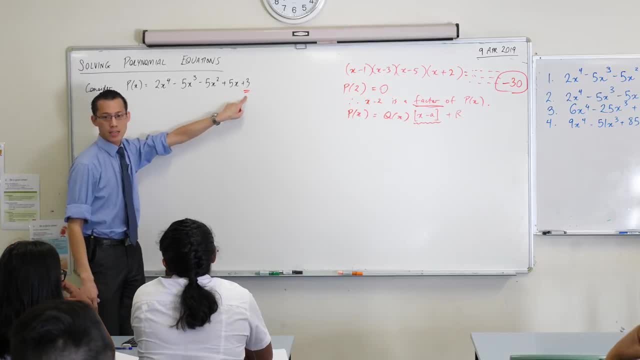 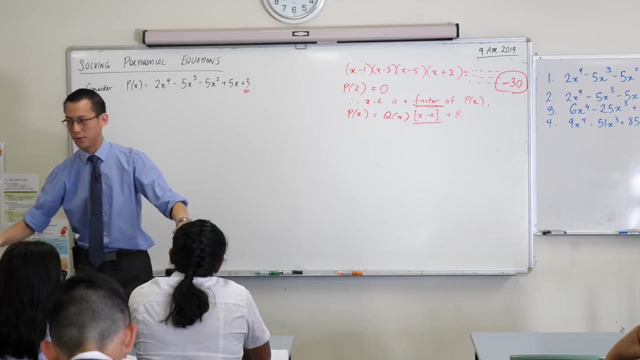 So I have a really good guess that either 3 or negative 3, if I put that in, I'm going to get 0.. So here's what I want you to do. You're mostly in pairs- Not every single one of you, but mostly. 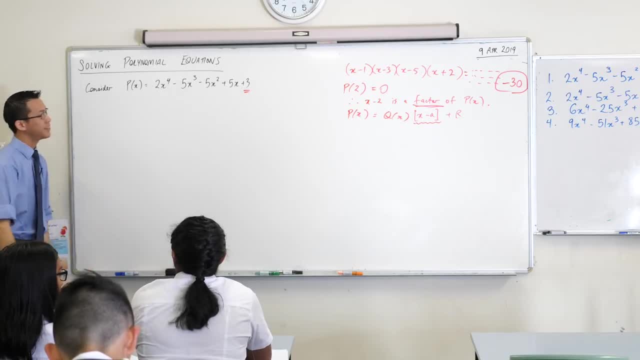 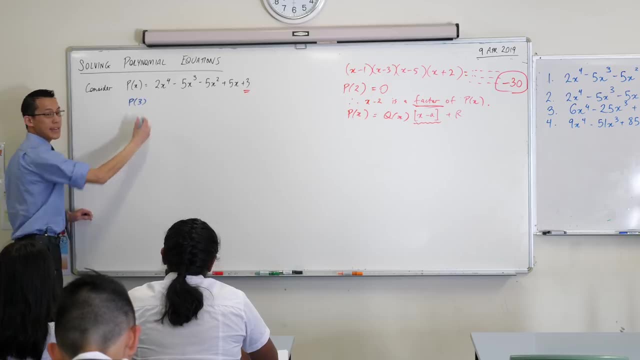 I want you to get your calculator out right now, and you'll need both of you to have a calculator. And what I want you guys to do with me is I'd like one person in the pair to test p of 3, and then I'd like the other person to test. 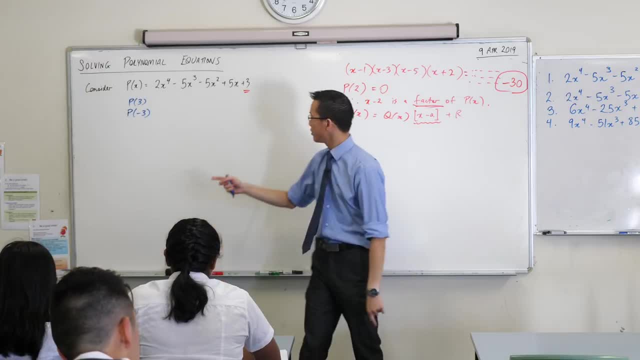 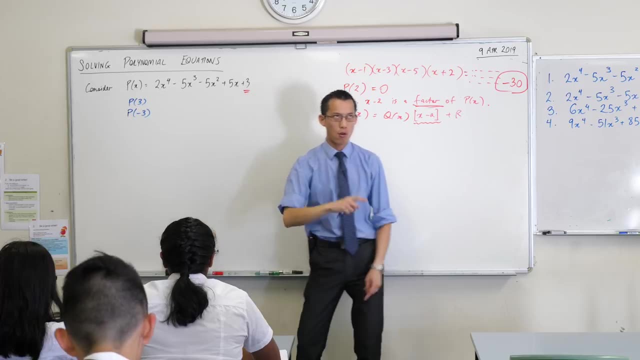 negative 3, okay. So what you're going to do is you're going to write all of this right, Even though you might know that negative 3 to the power of 4 is 81, right? You might actually know that. 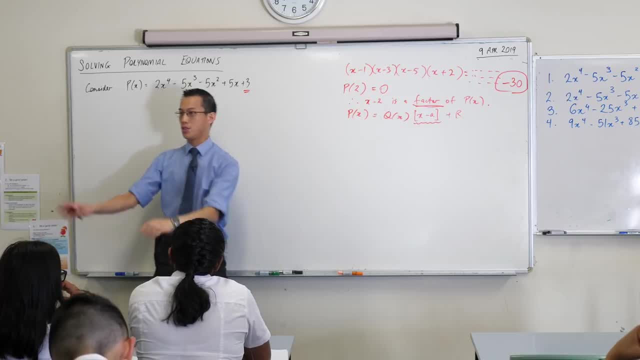 if I put that in, I'm going to get 0, okay, So here's what I want you to do. You're mostly in pairs, not every single one of you, but mostly I want you to get your calculator out right now. 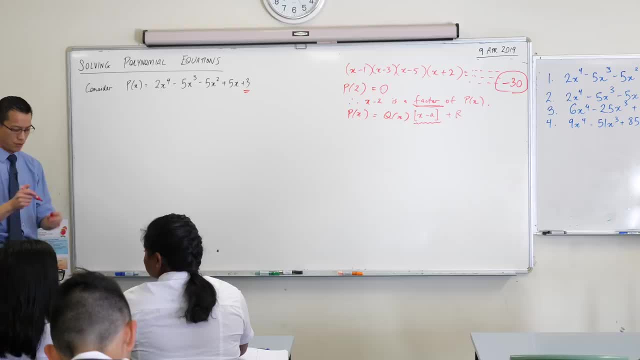 and you'll need both of you to have a calculator, And what I want you guys to do with me is I'd like one person in the pair to test p of 3, and then I'd like the other person to test negative 3,, okay. 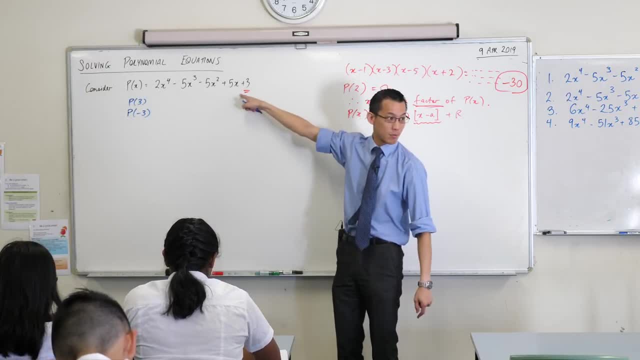 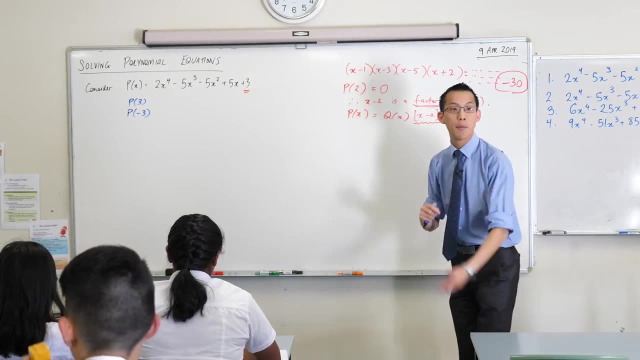 So what you're going to do is you're going to write all of this right, Even though you might know that negative 3 to the power of 4 is 81, right, You might actually know that You might be really good with your arithmetic. 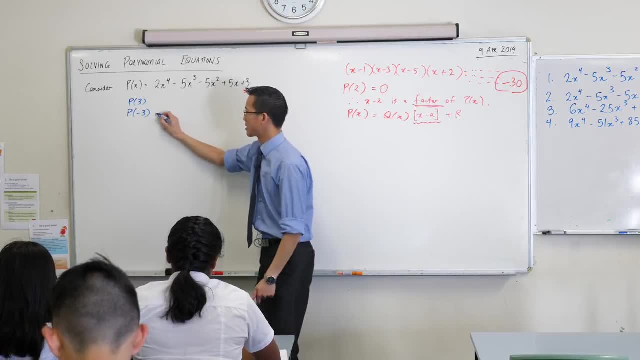 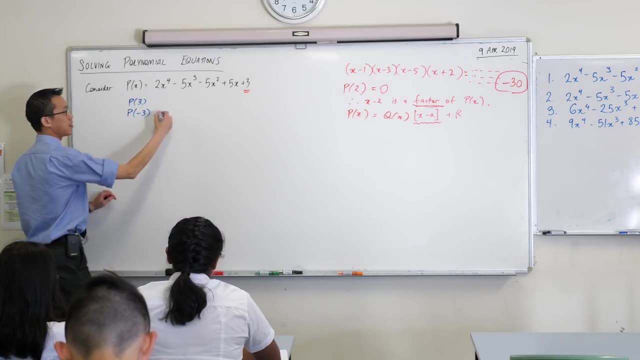 I'm actually going to ask you to put it into your calculator like this line here, with all of the substitution. That will make it easier for you to test other numbers if it so happens that this isn't the one that you wanted. So this is what for the negative 3 people. 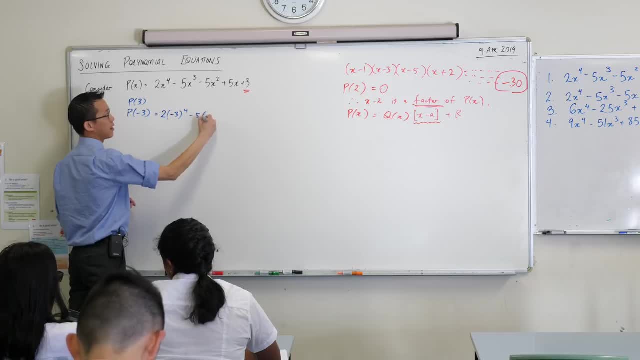 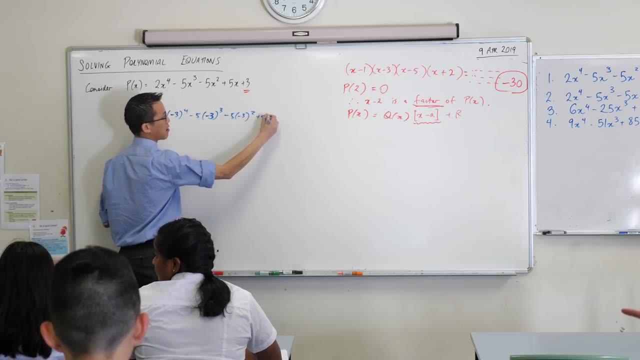 this is what you're going to be putting into your calculator display. So negative 3, it's a really messy 3.. So that is what you're going to be putting in, and with the p of 3,, you're obviously going to be putting in positive 3s. 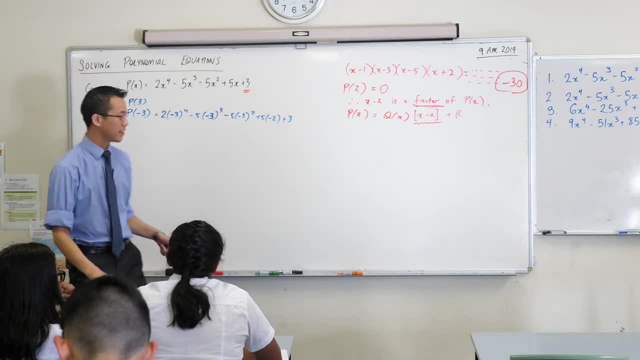 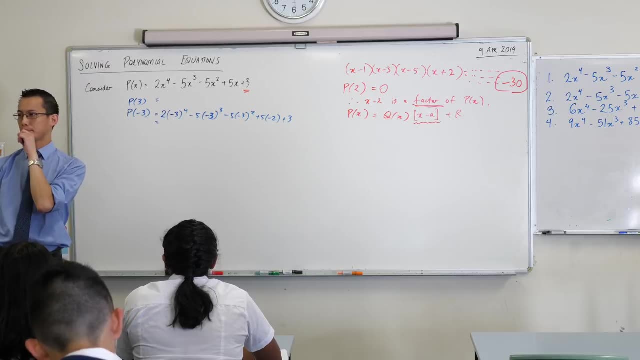 rather than negative 3s. okay, I'm going to give you a second. Okay, So who tested negative 3?? Hands up, Should be half of you, right Hands up, Okay. Okay, you're still getting there. 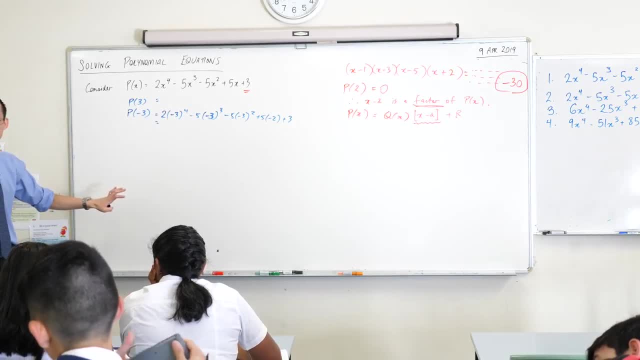 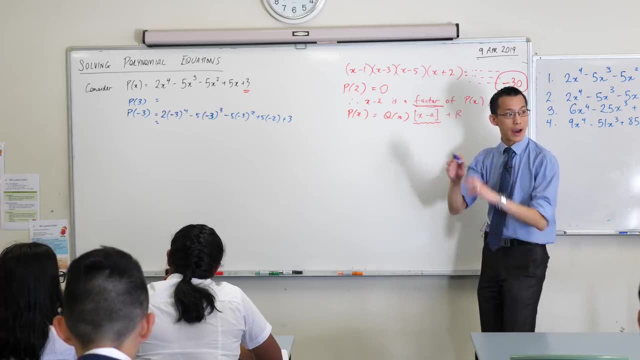 All right, I'll wait for you guys to all get there. Okay, Justin, you put your hand up right. What did you get as a value out of the end? Oh, okay, that's right. Who actually got there? 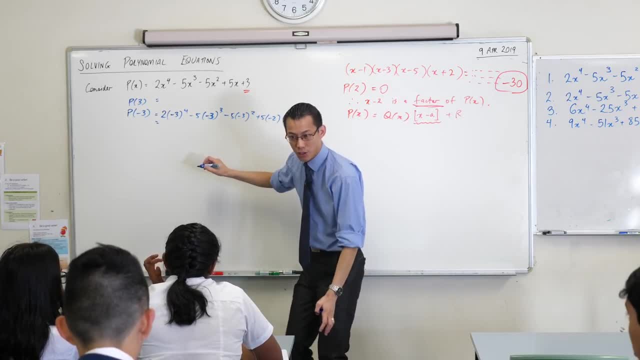 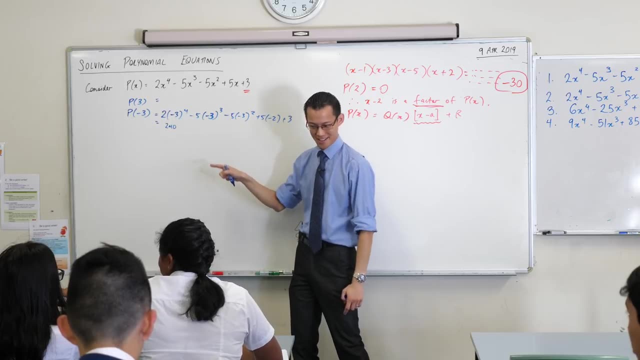 Yeah, go ahead, share with me Two, sorry, Forty 240.. Okay, so that's a big number, but that's not that surprising, because you've got these big 245?. Yeah, Maybe something's gone awry in here. 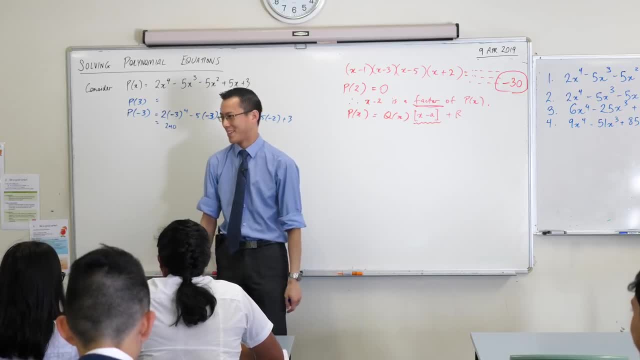 245,. do I have more concurrence there? 240.. Okay, guys, I'm going to have to rely on you. guys, You have the calculator in front of you. I'm like splitting that. No, no, no, I want you to do it. 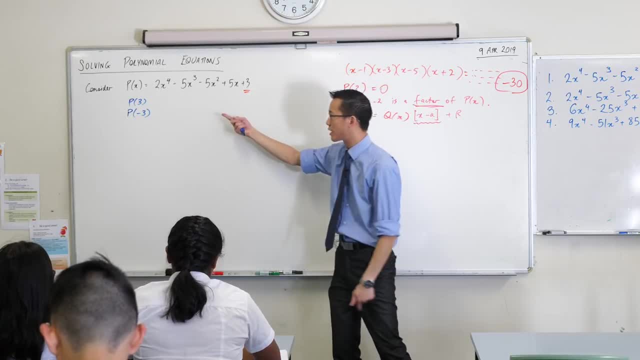 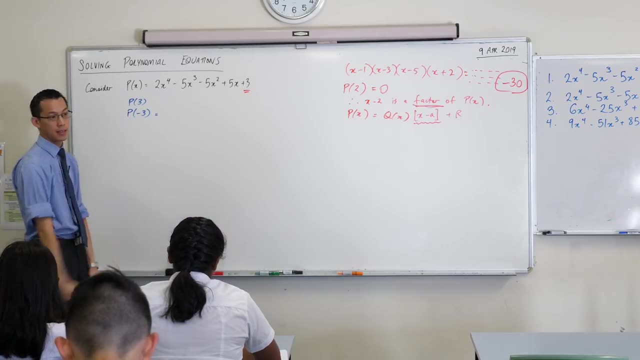 You might be really good with your arithmetic. I'm actually going to ask you to put it into your calculator like this line here, with all of the substitution. That will make it easier for you to test other numbers if it so happens that this isn't the one that you wanted. 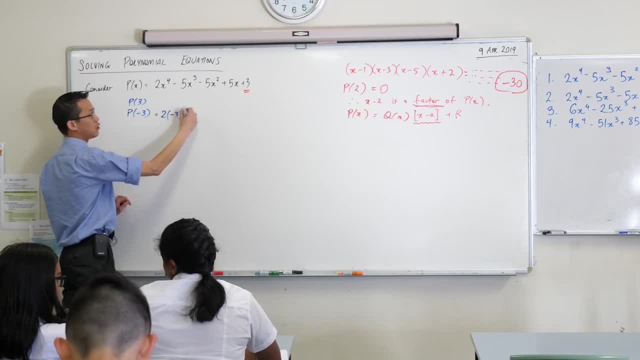 So this is what for the negative 3 people. this is what you're going to be putting into your calculator. This is what you're going to be putting into your calculator, So I'm going to display negative 3.. It's a really messy 3.. 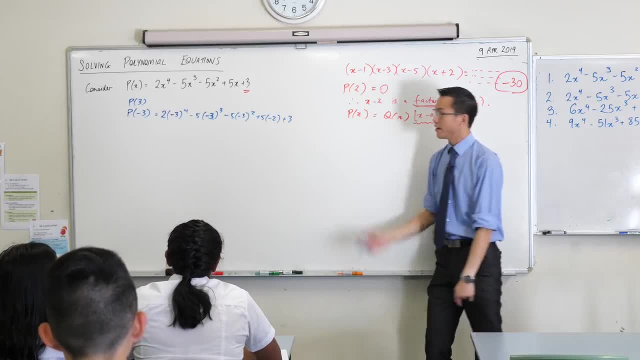 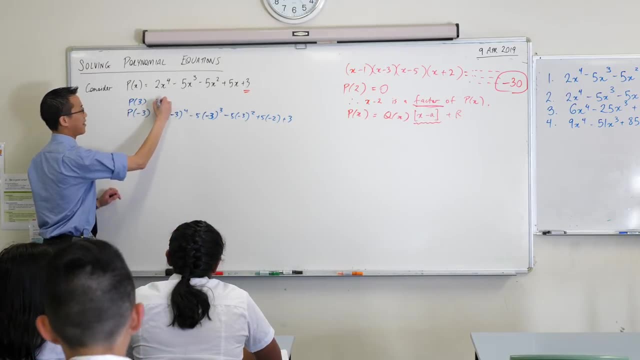 So that is what you're going to be putting in, and with the p of 3, you're obviously going to be putting in positive 3s rather than negative 3s. okay, I'm going to give you a second, Okay. 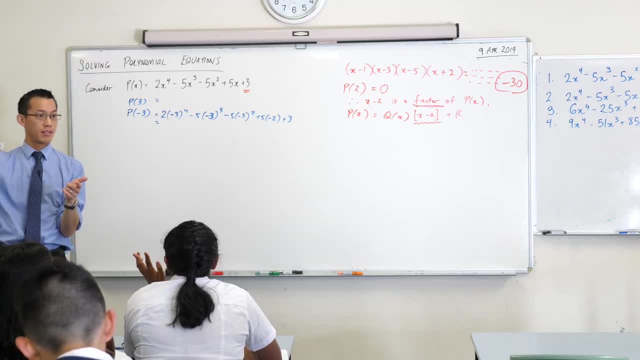 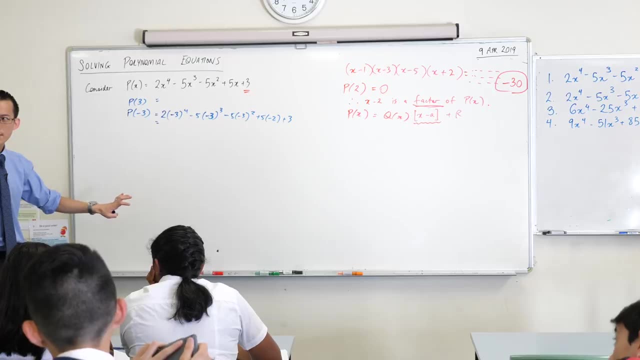 So who tested negative 3? Hands up. Should be half of you, right? Hands up, Okay. Okay, you're still getting there. All right, I'll wait for you guys to all get there. Okay, Justin, you put your hand up, right. 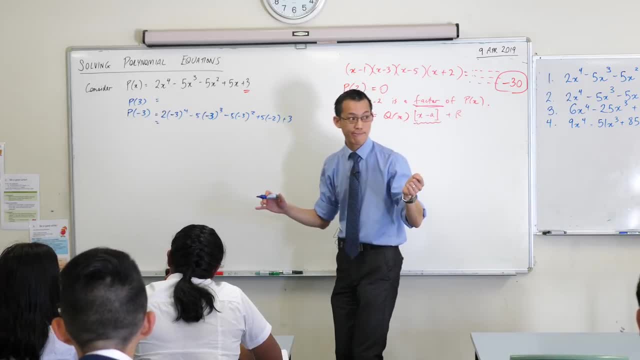 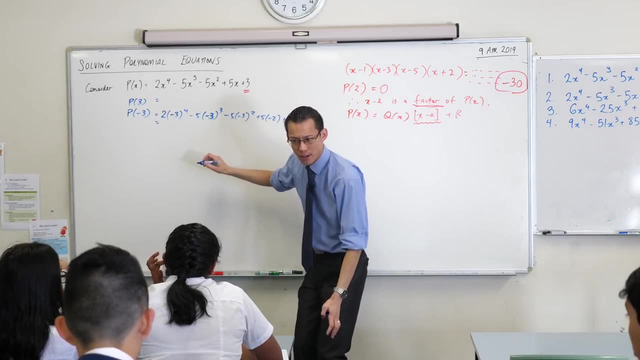 What did you get as a value out of the end? Oh, okay, that's right. Who actually got there? Yeah, go ahead and say it, Bobby: 240. Sorry, 40. 240.. Okay, so that's a big number, but that's not that surprising. 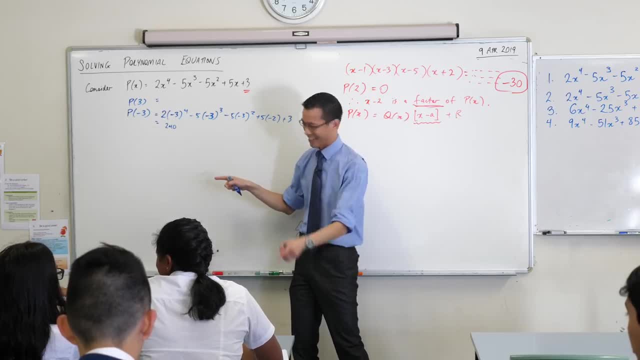 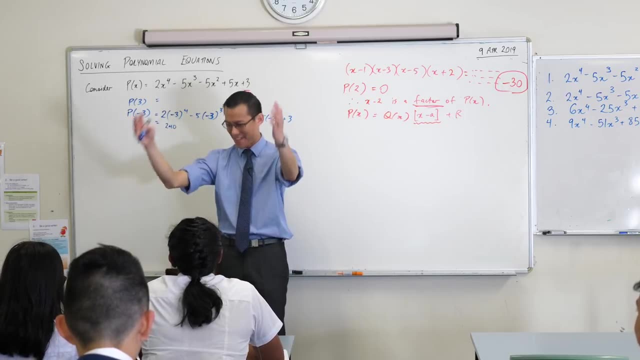 because you've got these big 245.. 245? Yeah, All right, Maybe something's gone awry in here. 245, do I have more concurrence there? 240.. Okay, guys, I'm going to have to rely on you guys. 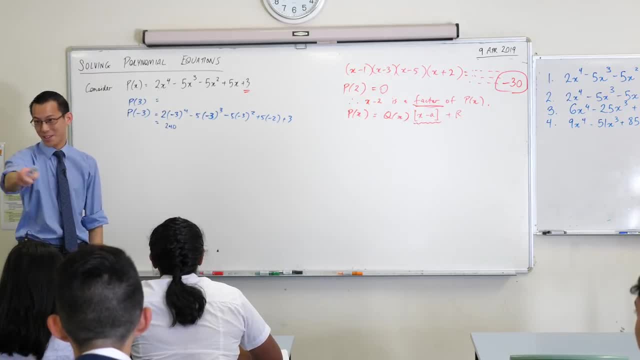 You have the calculator in front of you. I'm like splitting that. No, no, no. I want you to do it. You're doing it. I want you to do it right. 240.. 240, 245.. 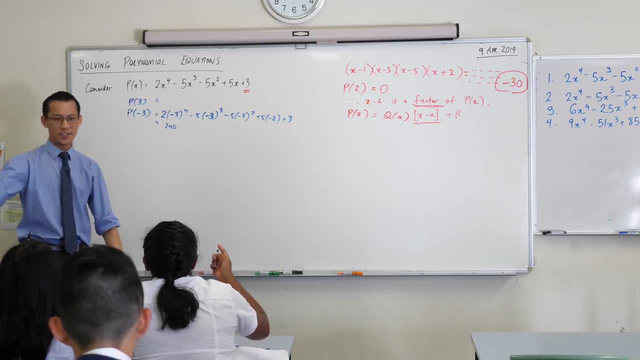 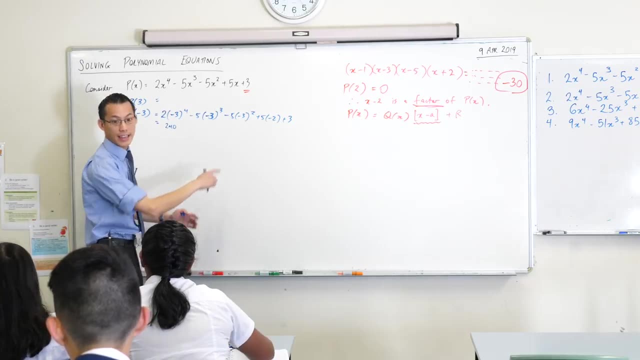 You're doing it. No, I want you to do it right: 240, 245.. I'm not playing you. I'm waiting for you guys to give me the answer. Say it again. What did I? Oh yeah, I did two. 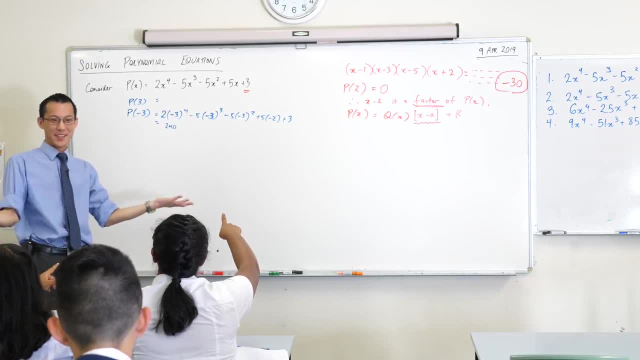 Sir, stop playing us. I'm not playing you. I'm waiting for you guys to give me the answer. Say it again: You put a 2 minus 2.. Yes, What did I? Oh, yeah, I did 2.. 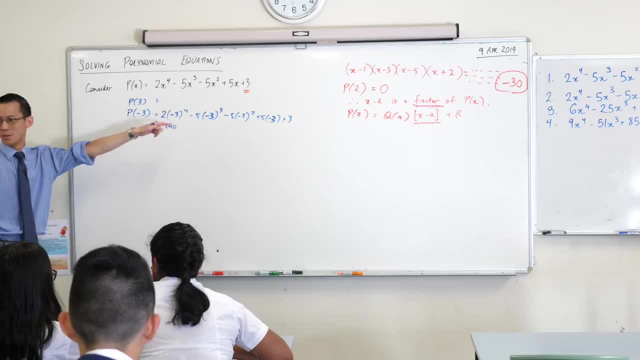 Thank you, So you're probably going to There's. What did I get? Was that the? Was that the end? Yeah, yeah, probably. Yeah, people just read my People read my wrong number on the board. That's hilarious. 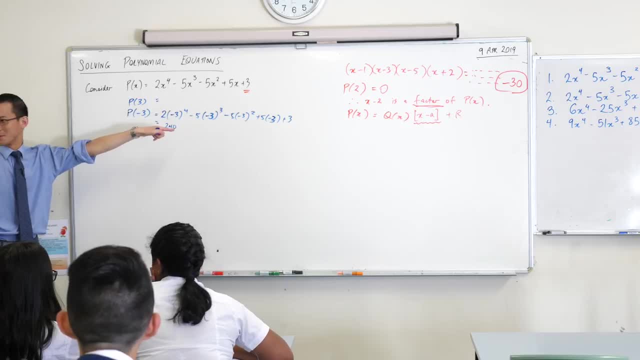 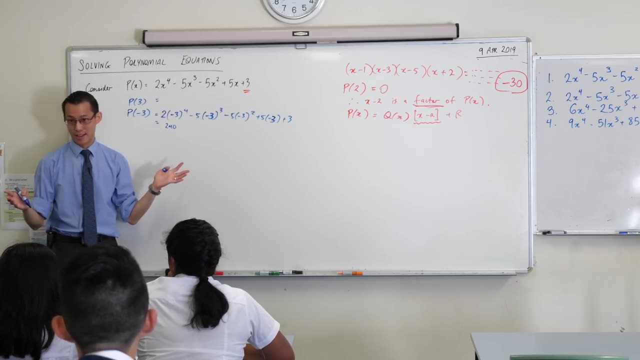 Thank you. Was that the Yeah? People just read my People read my wrong number on the board. That's hilarious, Okay, Have I got 240 then? Yes, Okay, fantastic. So what this tells us is, if I divided this original polynomial by: 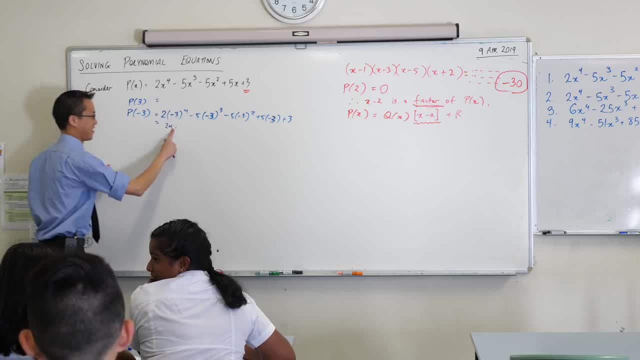 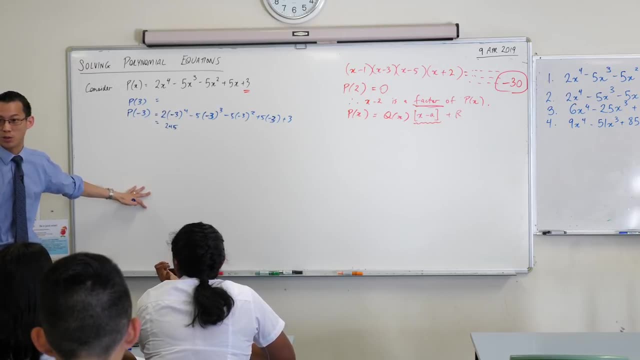 245.. Did you actually? It says 245 because, Oh yeah, All right, there we go. Okay, That's 240.. Do you notice why I'm not that actually interested whether it's 240 or 245?? What am I searching for? 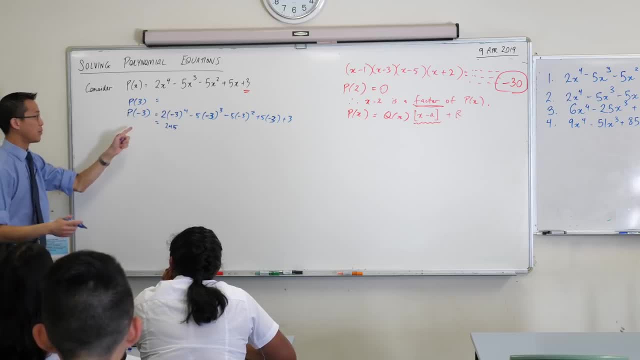 Zero. I'm searching for zero And I'm like it is neither of those. okay, Has someone already tested this? What did you get? Negative You got. You got zero. Okay, Now I could go straight to one of these. 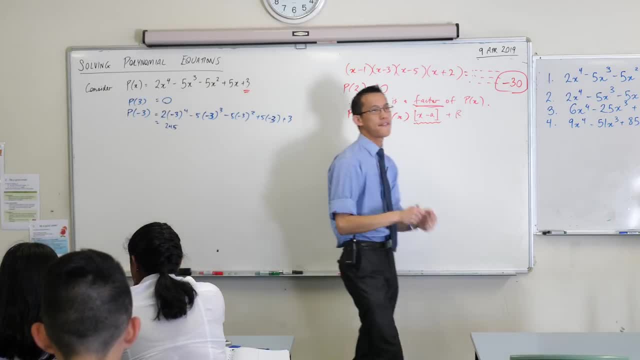 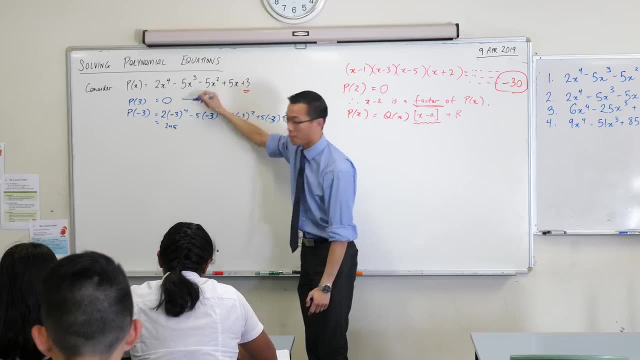 and know with reasonable confidence that one of them would give me a factor because of this number on the end here. right, This three, okay. So what I can say is: oh, from this line, if p of three is equal to zero. 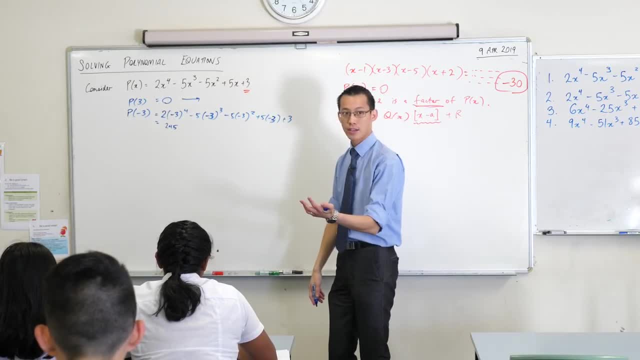 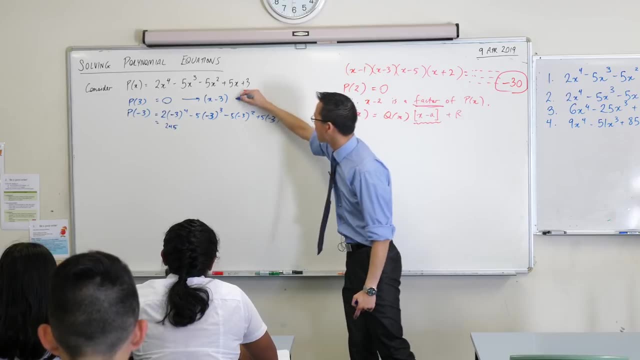 what can I conclude? X minus three, Very good. Yeah, Parham wasn't even here yesterday and he's followed the pattern right. X minus three is a factor, And so what I can do is I can divide this original polynomial. 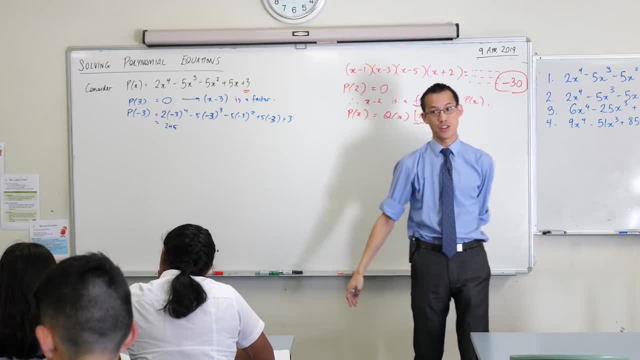 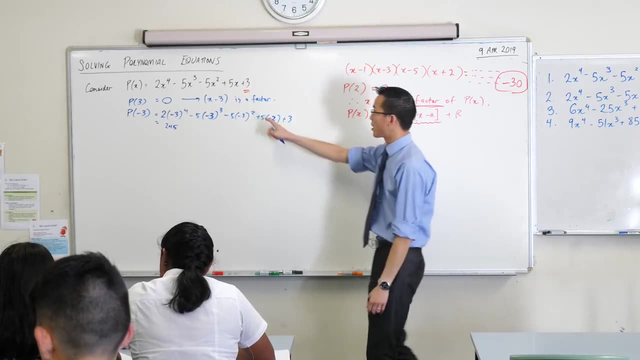 by X minus three, I will have to go to polynomial long division at this point, okay, But then I'm going to have something simpler and then I can work on that smaller problem. okay, Can I ask you guys right now: go ahead. 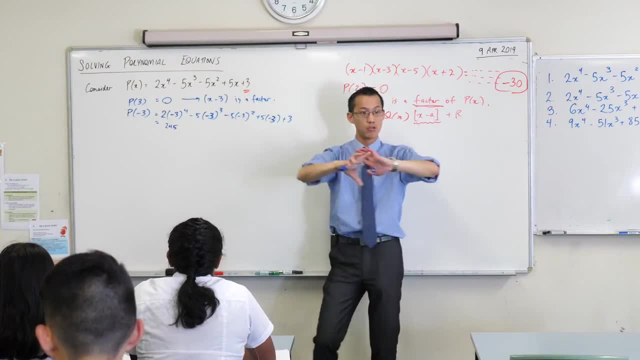 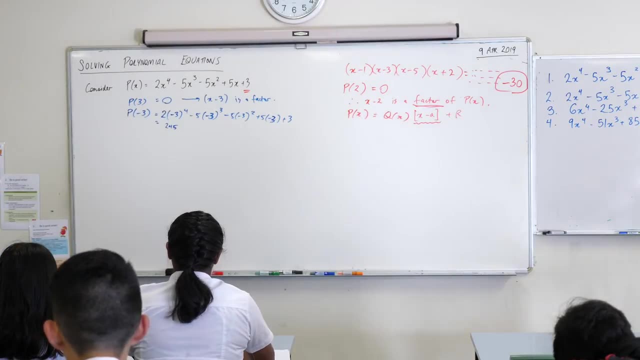 divide this big monstrous quartic by X minus three, do the long division. I'm going to give you a few minutes to do that. okay, Have a go. And then let's see if we get some agreement this time on the cubic result that we get. 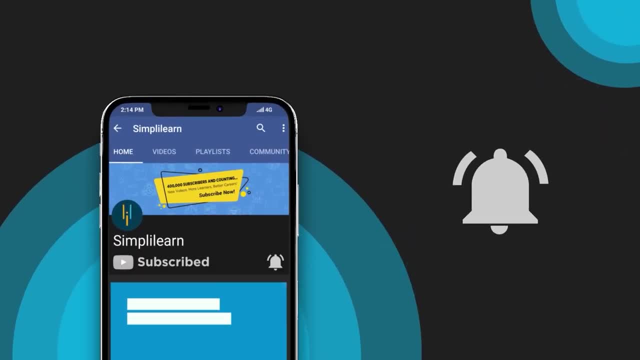 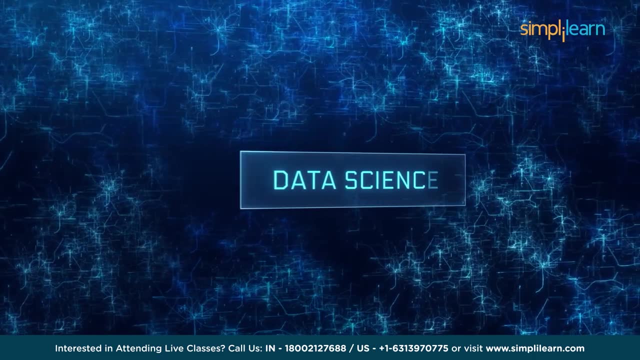 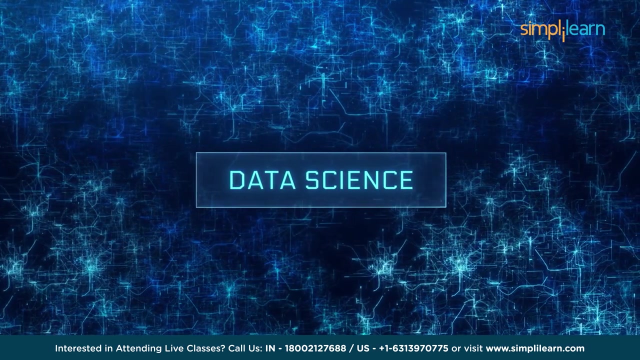 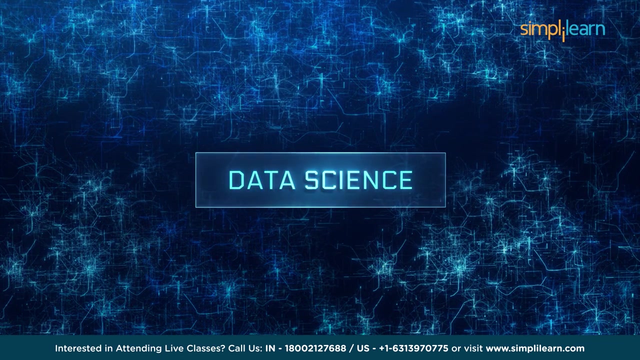 Welcome to the world of advanced data science, where cutting-edge techniques and advanced analytics converge to unlock the untapped potential of data. In this dynamic and transformative course, we will delve into the depths of the data universe, equipping you with the skills and knowledge needed to harness its power for groundbreaking insights and tangible 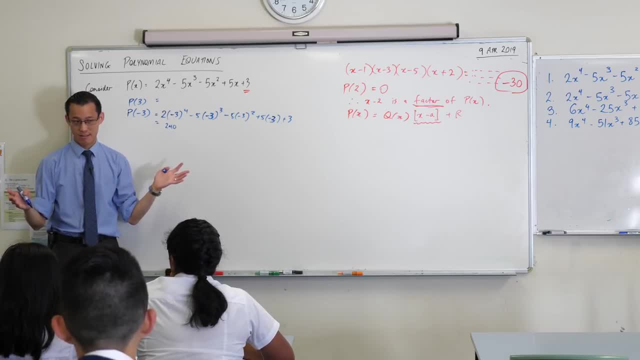 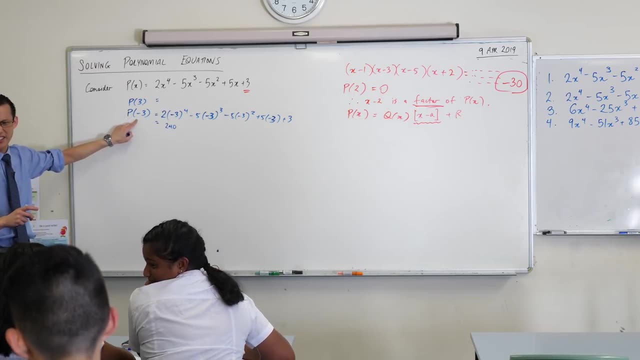 Okay, Have I got 240? then? Yes, Okay, fantastic. So what this tells us is, if I divided this original polynomial by 245.. Did you actually? It says 245, because, All right, there we go, Okay. 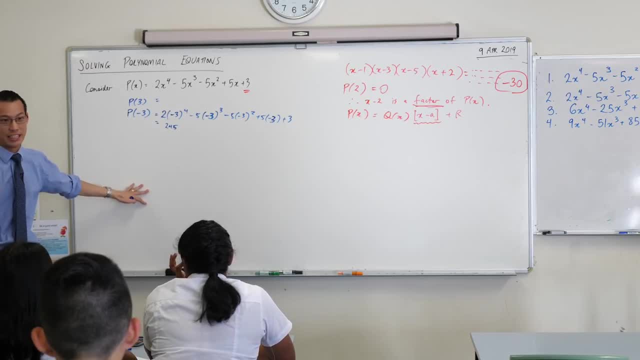 That's 240.. Do you notice why I'm not that actually interested whether it's 240 or 245?? What am I searching for? Zero, I'm searching for zero And I'm like it is neither of those okay. 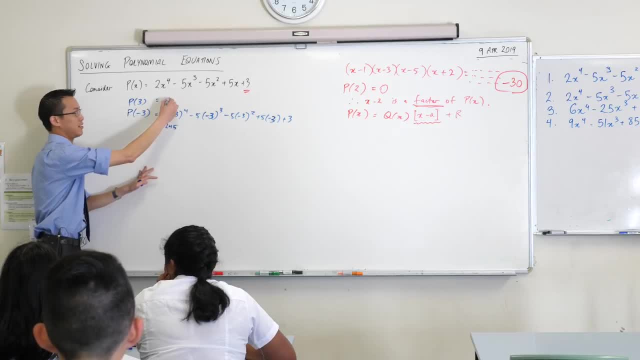 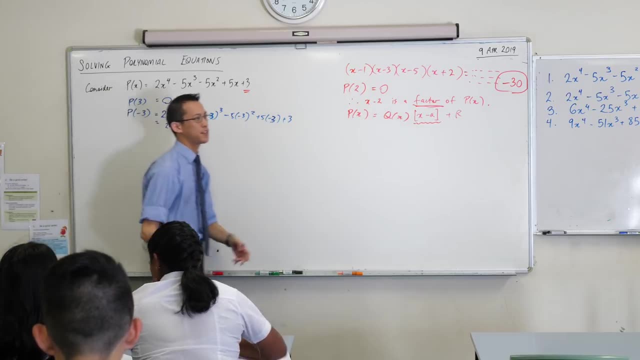 Has someone already tested this? What did you do? What did you get? Negative, You got zero. okay, Now I could go straight to one of these and know with reasonable confidence that one of them would give me a factor because of this number. 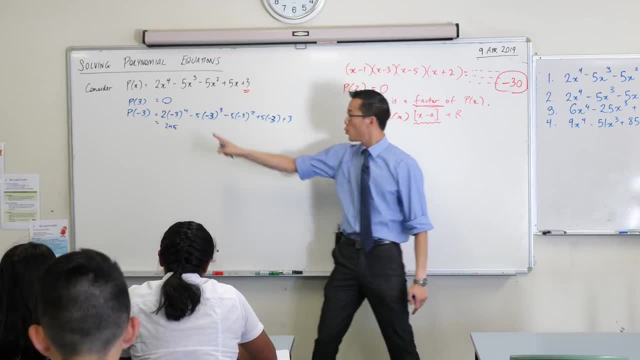 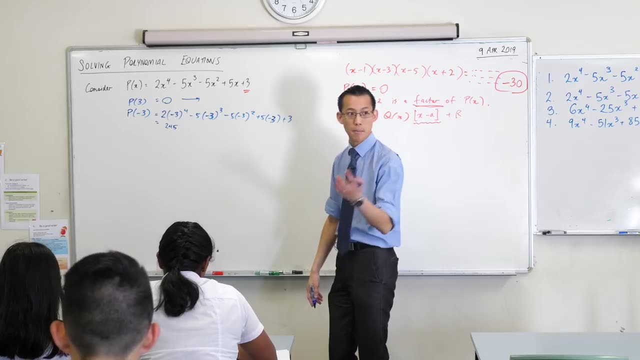 on the end here. right, This three, okay. So what I can say is: ooh, from this line, if p of three is equal to zero, what can I conclude? X minus three, Very good. Yeah, Parham wasn't even here yesterday. 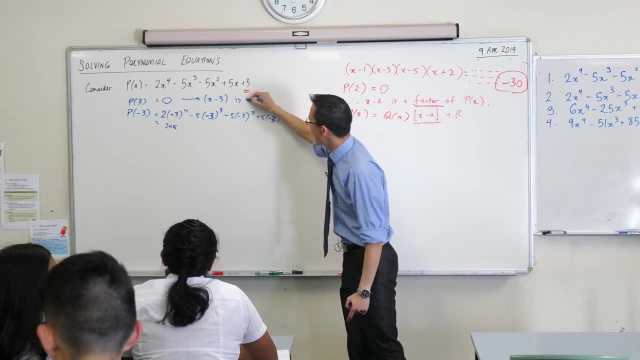 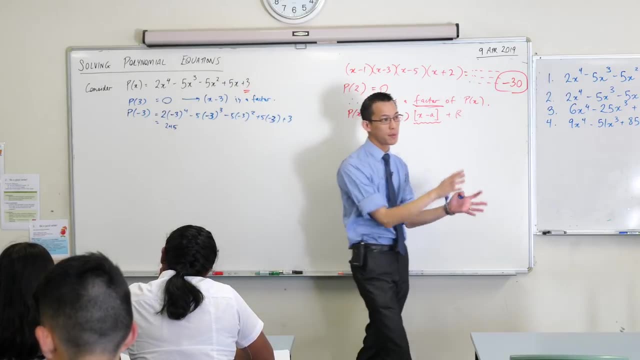 and he's followed the pattern right. X minus three is a factor, And so what I can do is I can divide this original polynomial by X minus three. I will have to go to polynomial long division at this point, okay, But then I'm going to have something simpler. 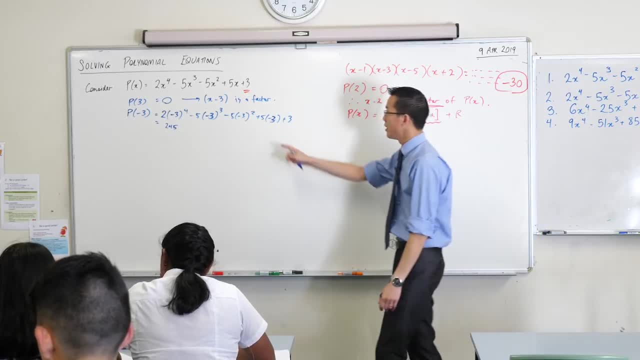 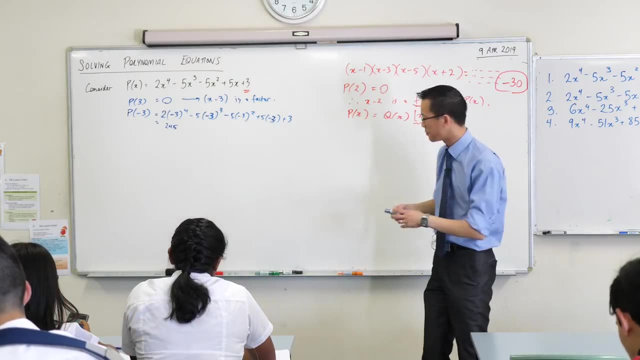 and then I can work on that smaller problem. okay, Can I ask you guys right now, go ahead, divide this big, monstrous quartic by X minus three. Do the long division. I'm going to give you a few minutes to do that, okay.